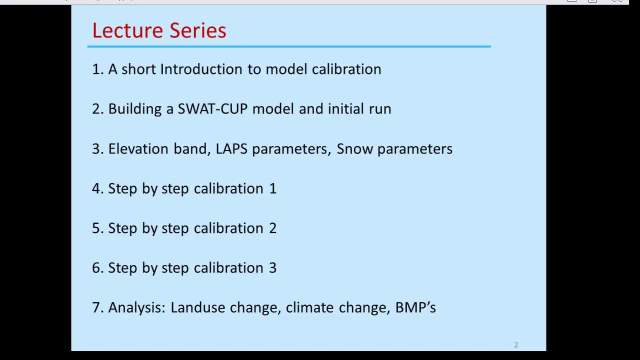 We continue thebeiining of complementCE2 approach. We will talk about the following steps. OK, so we have a patented, a modern model that calibrate different models, and then i may probably make some videos that show you how to analyze, now that you have created your calibrated model, what can you use it for? to you can use it. 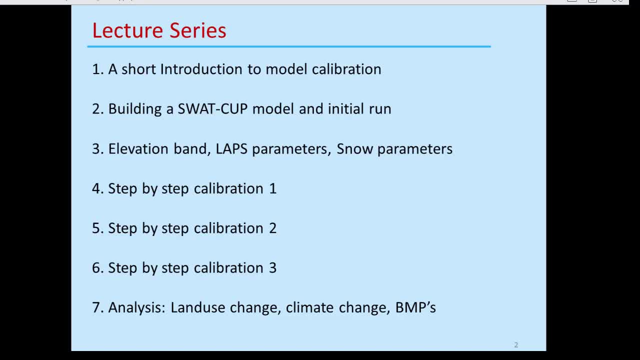 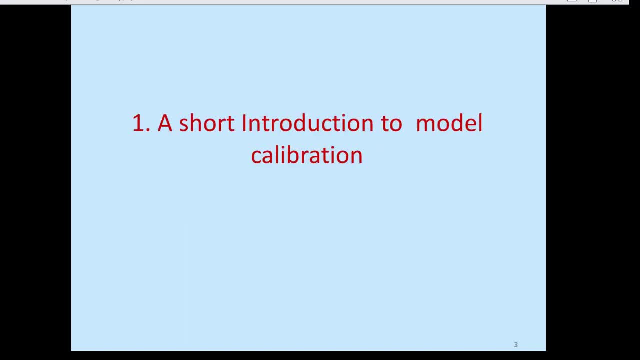 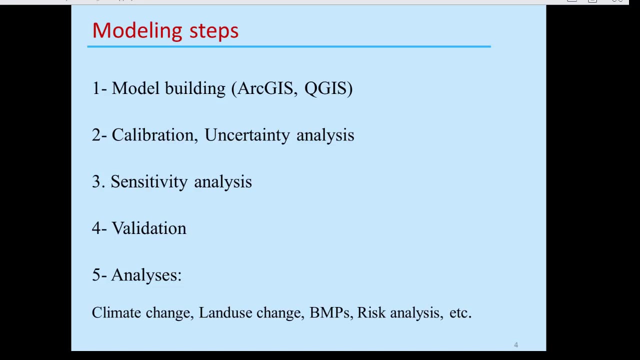 to analyze land use change, climate change, bmps and so on. we'll have some videos showing you on that. now let's get started with our first video, which is a short introduction to model calibration modeling steps. as you know, um, you have to follow several steps to build your model. 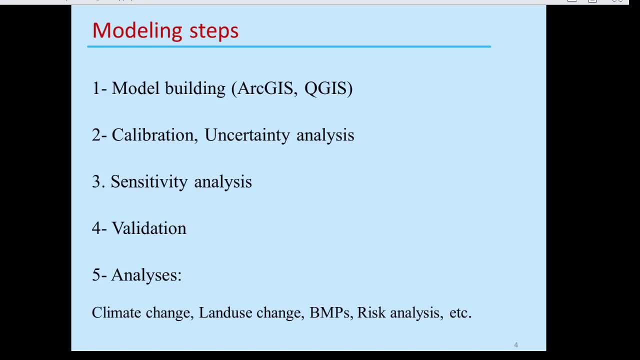 the first one being building the model in arc, gis or qgis. the next step is you need to calibrate that model, perform uncertainty analysis, validation, sensitivity analysis and so on, and then at the end, you may want to do some climate change analysis, land use change analysis, bmps risk. 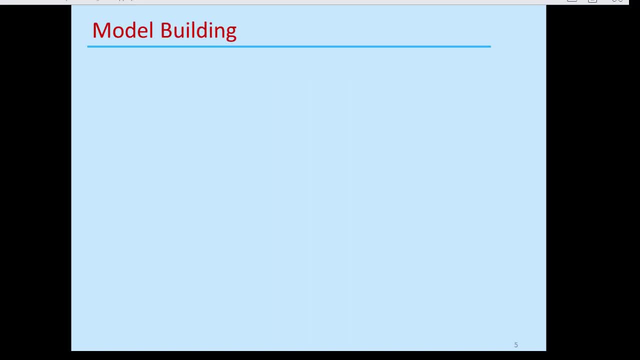 analysis and and so on, model building. so for swat, you build your model in arc swat or q swat. that is, you used arc, gis or qgis to build your model. at the end you will get a text in out folder, right? i'm not going too much into a swat model building- arc swat or q swat. once you have done. 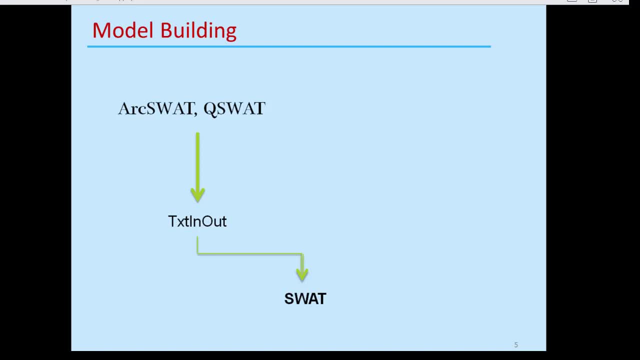 all that, you will get a folder called text in out which contains all the files that you need to run a swat model or the swat program. i should say swat is a fortran program and it uses text files to read the inputs, so it's really not much to do. 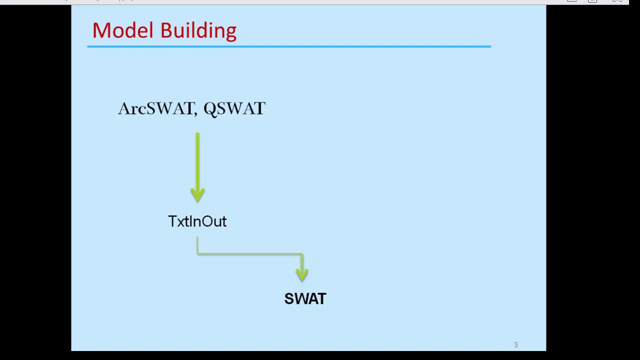 after you have built the model with arc swat or or q swat. on the other hand, swat cop um uses that text in out and then calibrates your model. your parameters at the end are in a file called parinf. so after calibration what you have, which consists of or makes up your swat model, is the text in out folder. 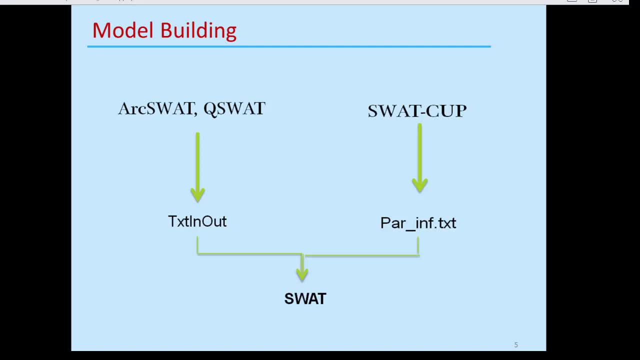 plus parinf folder. these two folder contain all the information that you need to run the swat model. often there are some form ofじゃ where the swat model is generated. is it sql that we used in the previous step? so here you see our model, altering the swat model after it is made a multi folder. 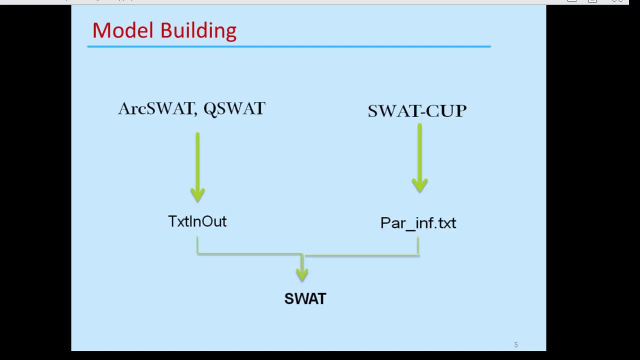 we were able to import px and png images in this chapter, so we take some data and put them into this template and i'm going to show you how that work here. so in a second, to see if the model as it does, they are saved to a. we have aается very shortуйте e suite. that Table eleg doesn't give us the. 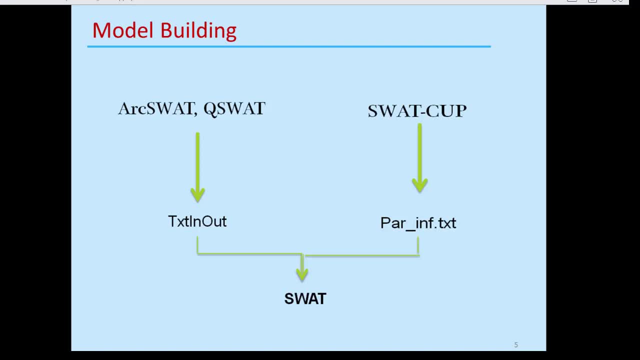 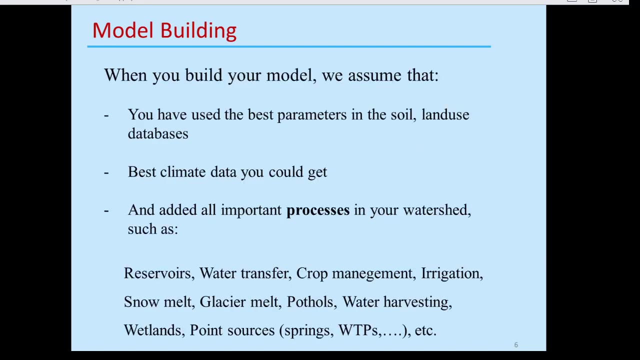 time. okay, Banko, right now iга program independent of ArcSWAT or QSWAT or SWAT, that it's a standalone program that tries to calibrate your SWAT model. Now, when you have built your model- when you build your model, we assume that you have. 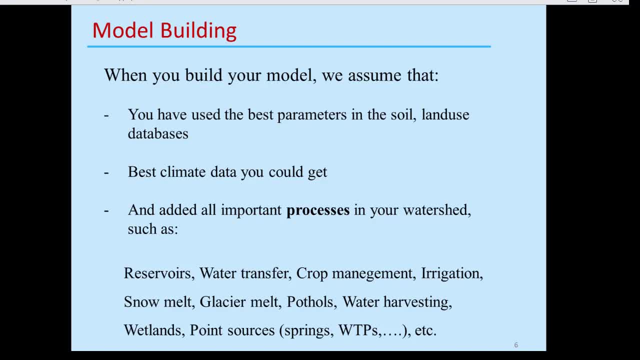 used the best parameters in the soil land use database, you have used the best climate data that you could get and you have added all the important processes that occur in your watershed in your model. By these processes I mean the reservoirs, water transfers, crop management, irrigation. 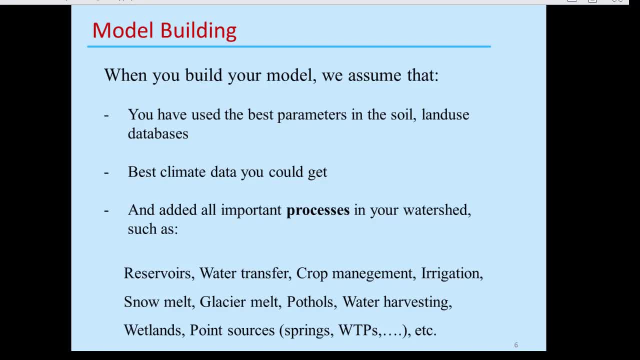 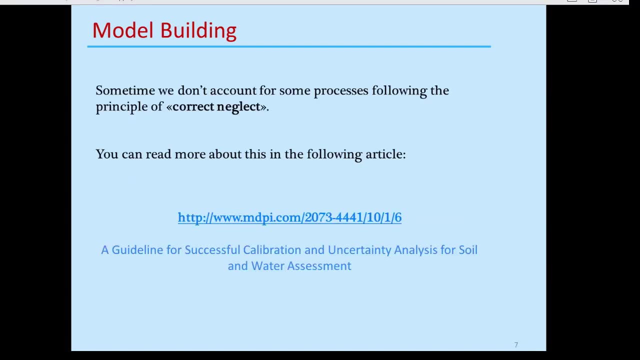 snow melt, glacier melt, potholes, water harvesting, wetlands, point sources such as springs and water coming from water treatment plants, and so on. Now model building, sometimes some of these processes- we don't account for everything that happens in the watershed. 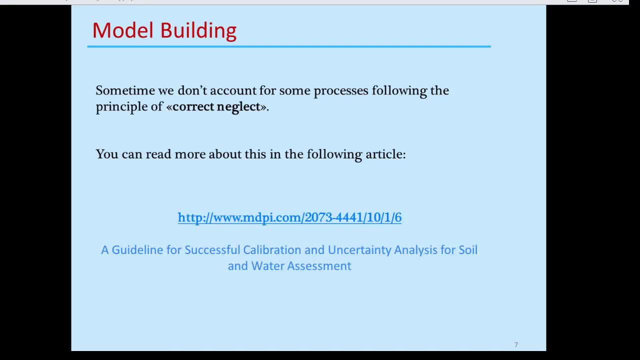 There is a principle called the principle of correct neglect, where you neglect the processes which are not important or of any consequence in the watershed, But processes that are important and of consequence. they should be, of course, included in your model. Now you can read more about this in the article which is listed here. 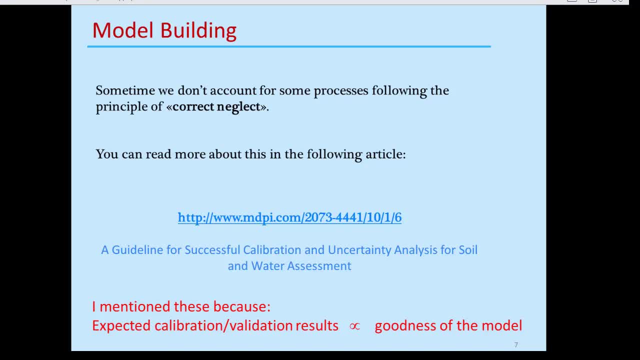 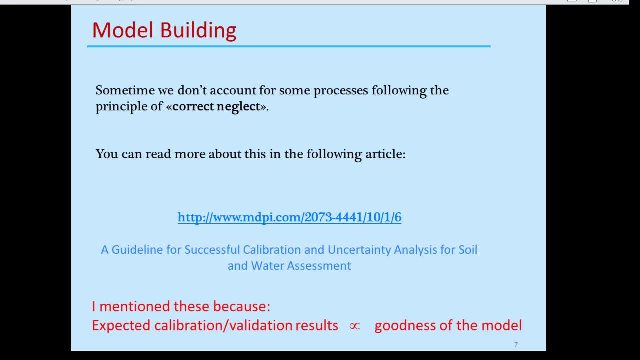 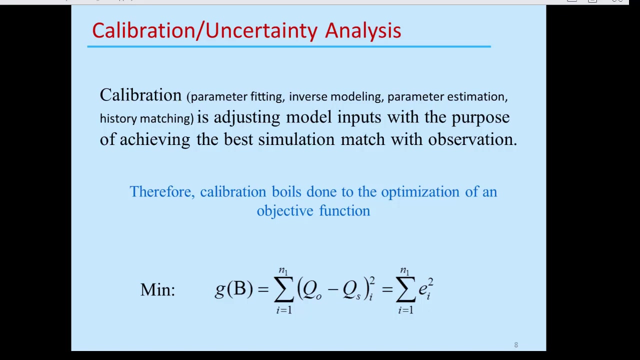 So you cannot expect a perfect calibration result when you have not included, for example, important processes in your model or your data is really poor. So your expectation should be proportional to the goodness of your model. Now let's begin by discussing about calibration. 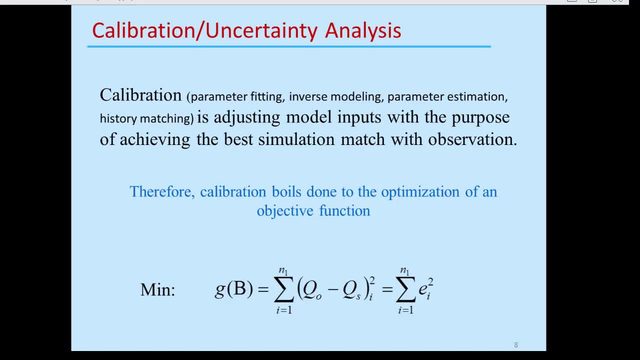 Calibration or uncertainty analysis. Calibration has many names. in the literature It's called parameter fitting, inverse modeling, parameter estimation, history matching. They all mean the same thing, which is calibration, And it is just theoretically very simple. You try to adjust your inputs so that you come your model simulations are the closest. 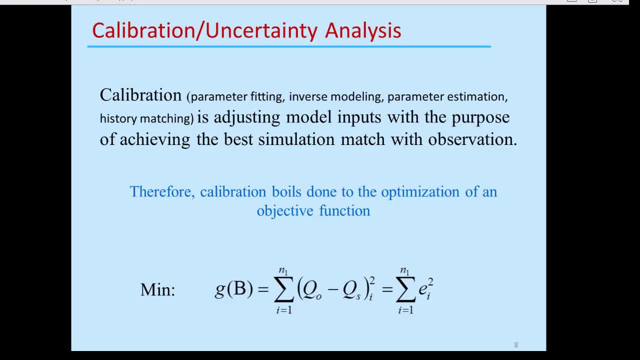 to the observation. So eventually, at the end, this calibration process boils down to optimization of an objective function such as the one here, that says you want to minimize the objective, your objective function, which is a function of the parameter set B, which tries to minimize, right the 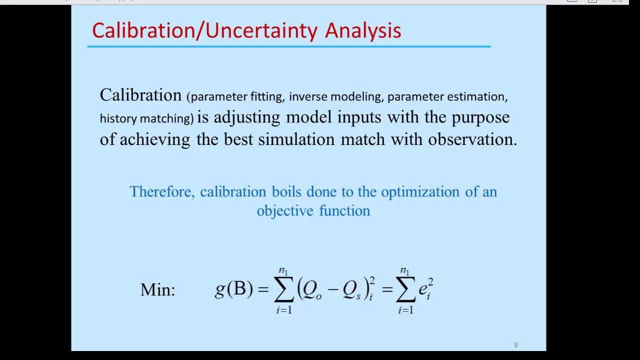 difference between observed, for example, discharge and simulated discharge. So this is an objective function that you try to minimize. Once you have minimized this, then you can deduce that the parameters that you obtained are probably the parameters that you're looking for. if the calibration, if this value of objective 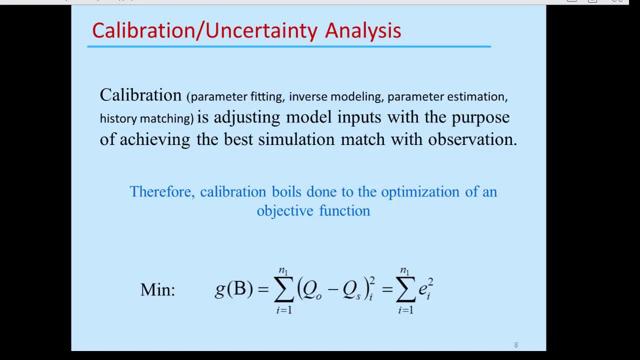 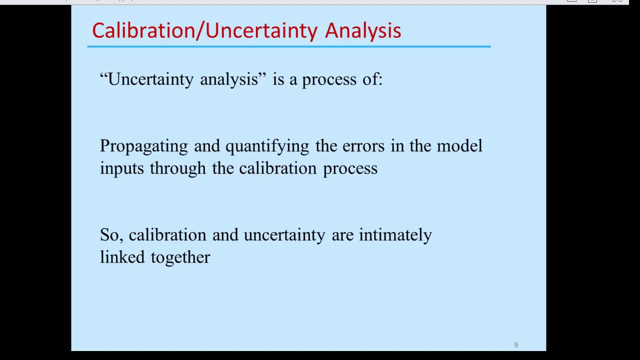 function is in this case small enough. Now, uncertainty analysis is therefore the process of propagating- Okay- And quantifying the errors in the model, model inputs or processes and so on, through the calibration process. So calibration and uncertainty analysis are really intimately linked. 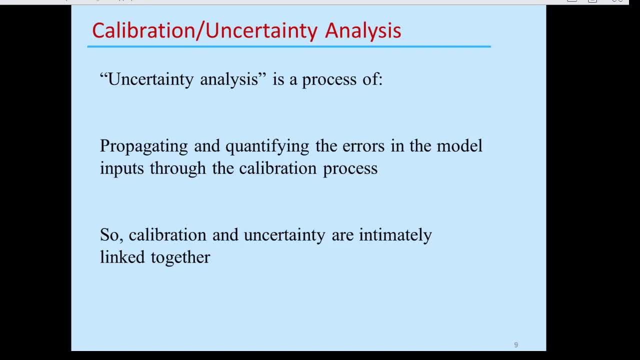 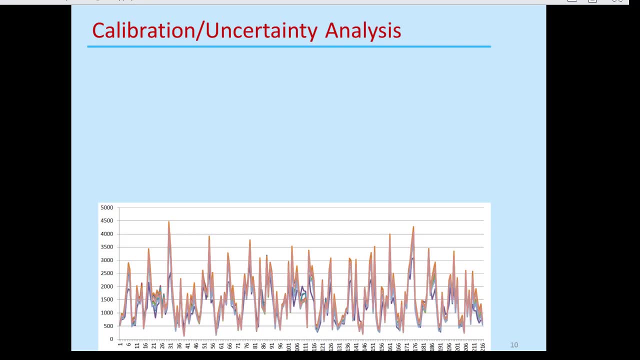 You cannot separate these from each other, And the reason for that is that, if you look at these graphs, there are 11 discharges here, So you can look at the data from 11 different data parameters, 11 different parameter sets, which are shown here. 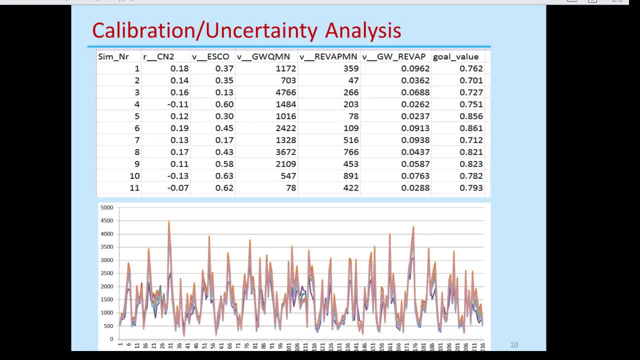 So you have 11 simulations. These are the different parameters. This is the value of the objective function. It's very close to each other. In fact, statistically they are not different from each other. If you look at the parameters, they can be quite different. 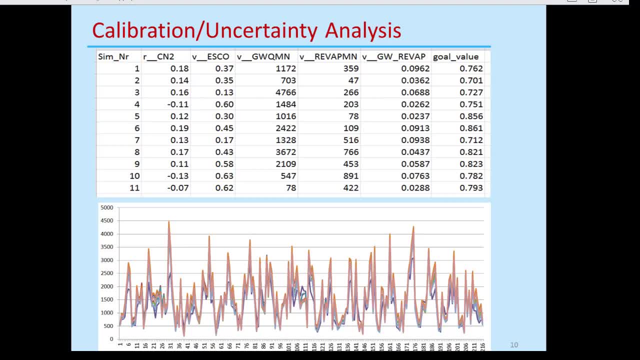 They can be quite different from each other. They can be quite different from each other, Okay, Okay, from each other. so the whole idea behind uncertainty is that you can have very many different parameter sets that give you the same result. statistically, the same result. so here the best simulation that everybody is after, the best. 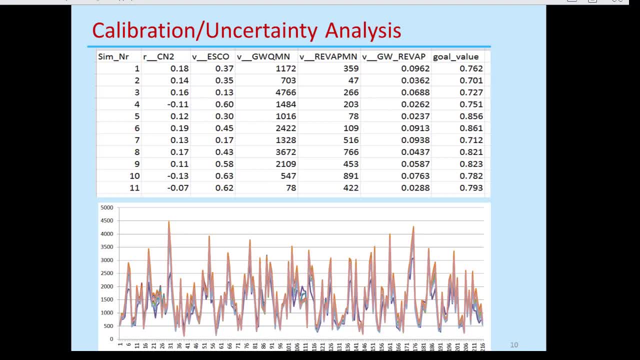 simulation. the best simulation has these parameters. now there isn't really a big difference between the best simulation and the next best best simulation or the next best simulation and so on. that's where the concept of uncertainty comes from. so if you have one good calibration result for your parameter, then you have. 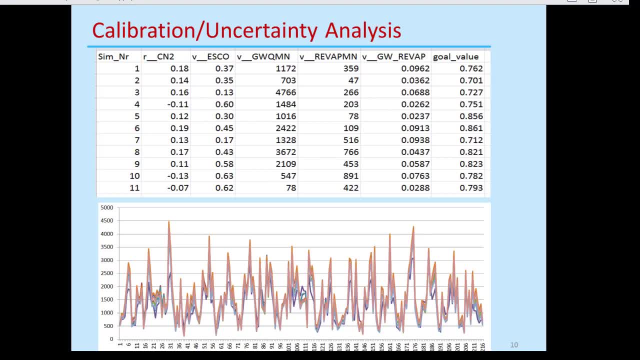 thousands of good calibration results for your parameter so you cannot pick one of them and say here is my result. so the idea that many of you have that now I want to put the best parameter set in the next best simulation so you can double prevent me from buying assistants at the right time, and you shouldn't. 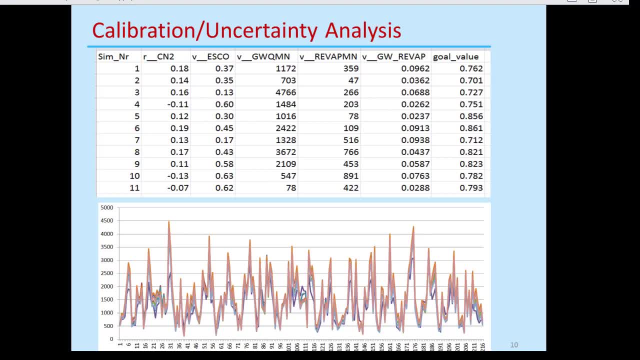 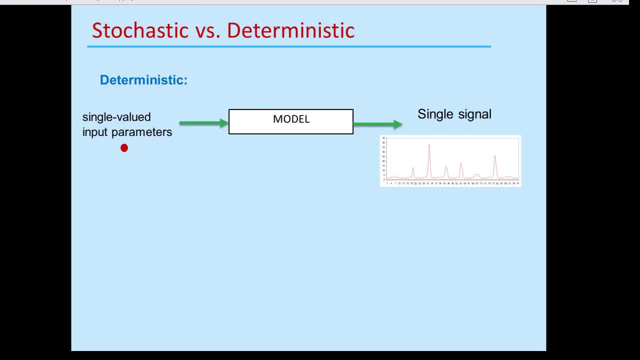 buy a particular model. so, as you can see the data from a Bank analysis, I think that the best model and the cause for this problem is in the next generation. so let me also show you what a basal simulation offers. is a sample of such a basal model. so below I have an example here: a hopes design SAM app from a. 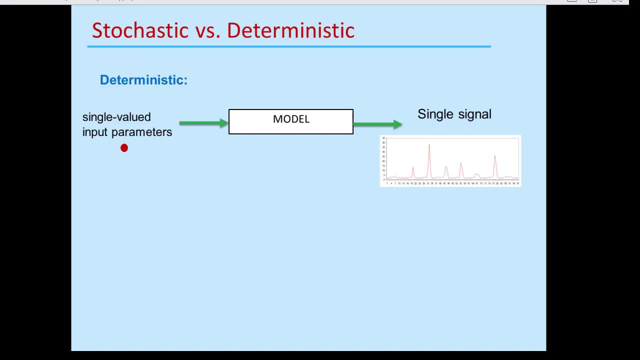 source tool, which I don't have exactly this information that I am going to share. but you see, this method and you can determine between ap那个 edition, me, And the model gives you a single signal of output, like discharge and so on. All models are deterministic. 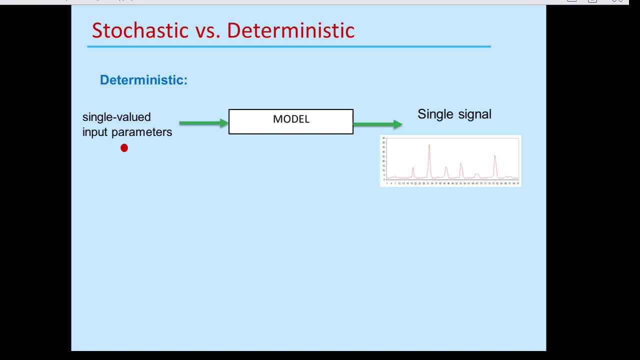 They take one value for a parameter and they give you one signal, But the minute you want to go the other way around, that means you want to use your signal like discharge and get your parameter back, which is the process of calibration. 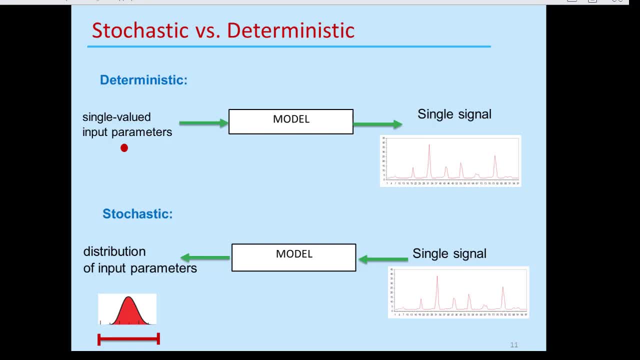 Calibration is what it does. is takes your output from the model and tries to find out your observation, and tries to find out the best parameter. The minute you go the other way around, the process becomes stochastic and you no longer get a single output from this approach. 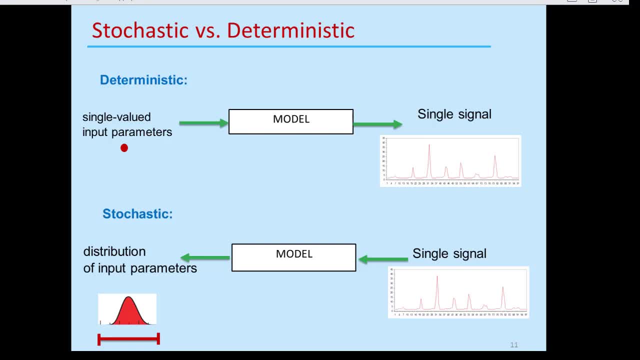 but you get a distribution of outputs or a range. So in this case the output would be our parameter. So parameters always have a range. when you are doing calibration, They are never a single value. No calibration program can give you a single value. 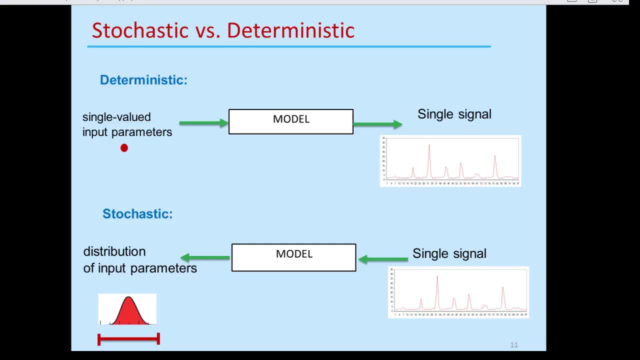 It can, but it won't be correct. You've got to consider the distribution in your output, which is the uncertainty of your model. So you have to carry this uncertainty in whatever analysis that you do with the model- And you should- You should not try to get the best, whatever that means. 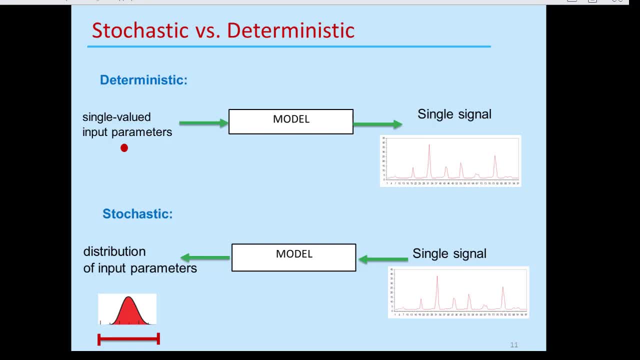 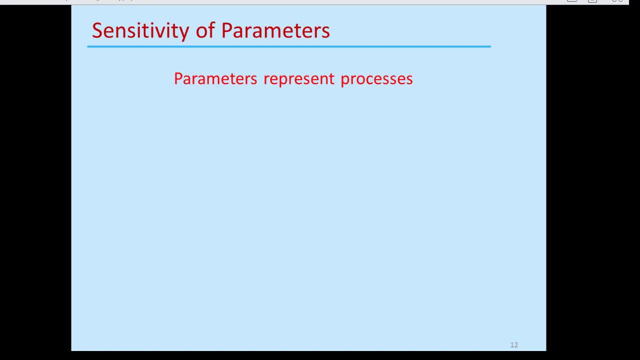 the best fit and then use only those parameters. Now next, sensitivity analysis. The sensitivity of a parameter. why are we interested in sensitivity analysis? It's because parameters represent processes. So the reason I'm interested in the sensitivity of this parameter. 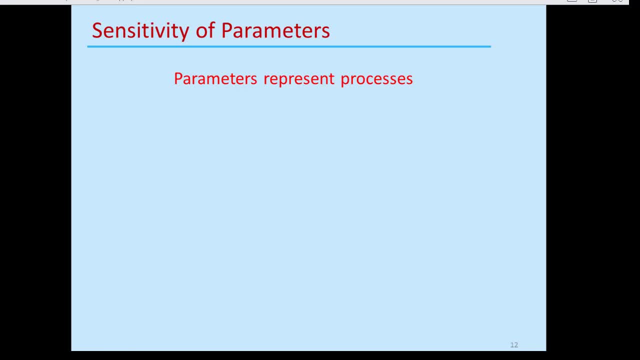 because this parameter represents a process. I'm actually interested in that process to know what are the important processes in my watershed. So sensitivity determines which process is dominant in the watershed, And for that we determine the significance of one or a combination of parameters. 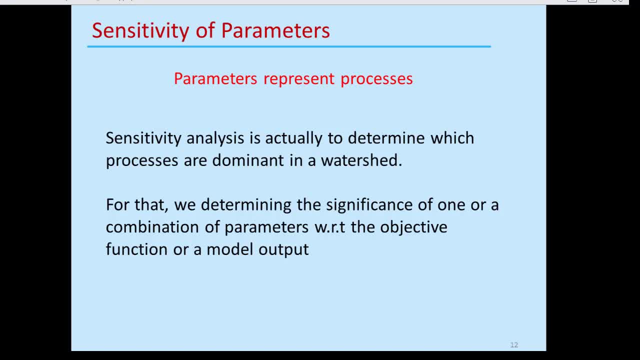 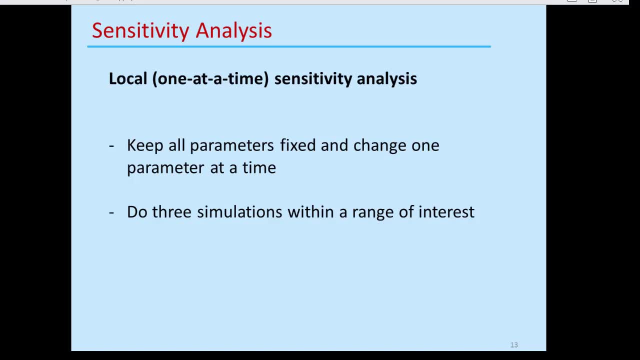 with respect to the objective function. Now there are two different methods for sensitivity analysis. in SWAT-COP There is a local or one-at-a-time sensitivity analysis. In this type of analysis we keep all the parameters fixed constant and change only one parameter at a time. 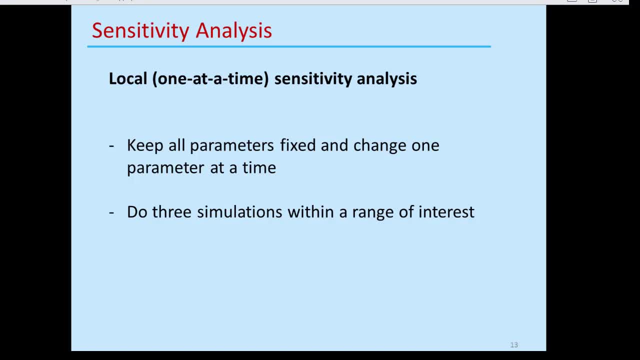 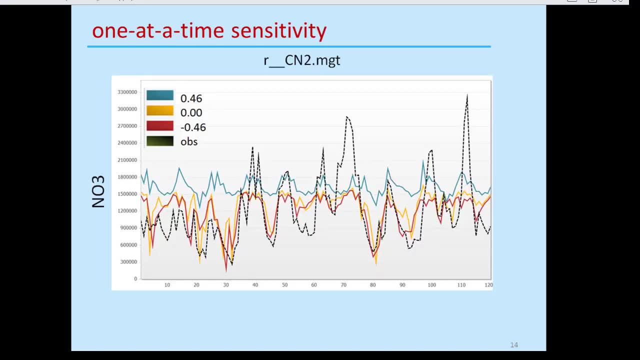 So, to determine this, what you have to do is you make, very simply, three simulations with a range of interest of your parameter and you look. you see how they look like. So in this case I'm using CN2, and with respect to nitrate, 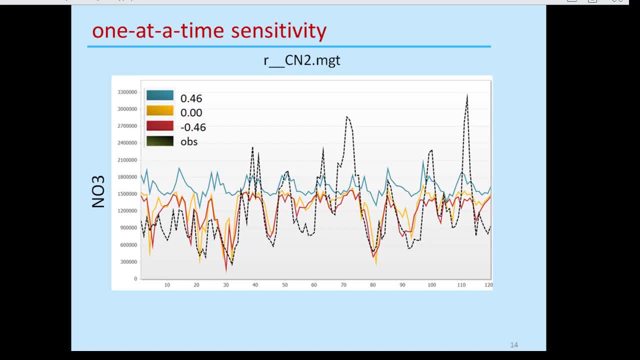 So I want to see how sensitive CN2 is. when I'm looking at nitrate, I do three simulations. I'm going to do three simulations with these three values of CN2.. The black dash line is my observation and this is what I get. 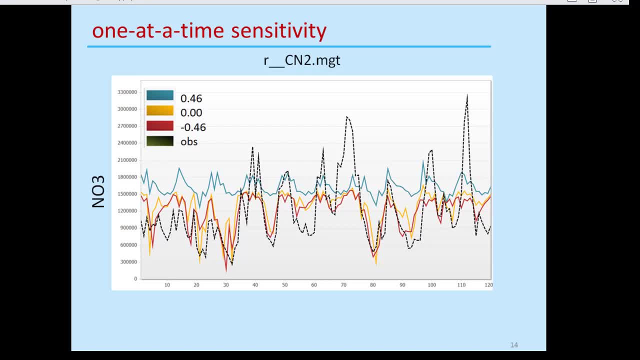 So from this I deduce that, first, CN2 is a sensitive parameter, because every value gave me a very different result, And, secondly, I can use this information to get an idea of the range of the parameter Right, The parameter range, the range of CN2, many people ask me initially. 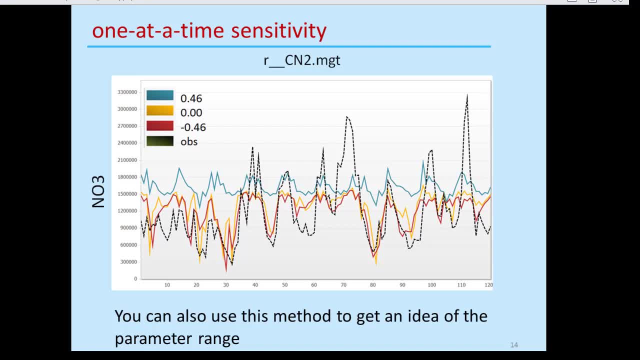 what should I use for range of parameters? Well, this is one way you can use to set the range on the parameter is that you do a one-at-a-time, a local sensitivity analysis within a range, and then you look at your results. 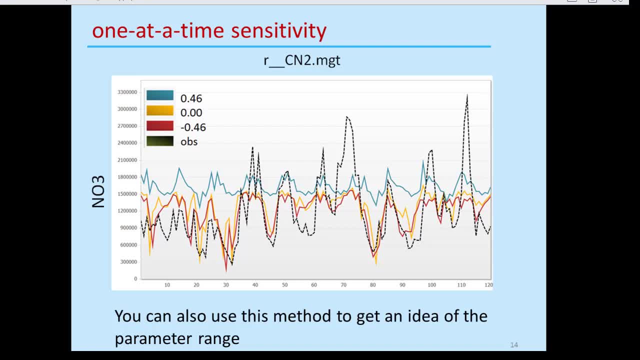 Now, when I look at this, it's clear that the best values are here, are down here, right? This 0.46 is up here and the other two values have this range down here. So clearly, I would like to be within the range of 0 to minus 4, 0.46. 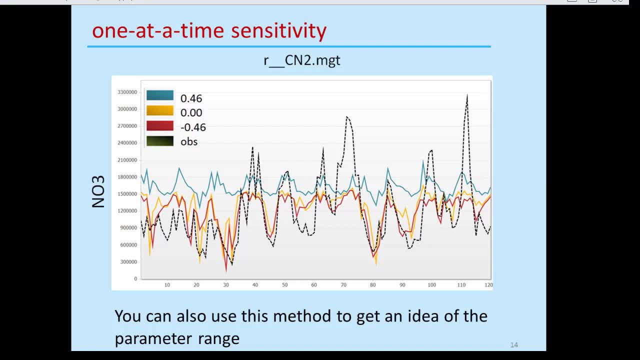 Now there are some observed peaks which I have to find other parameters that would fit those peaks. But as far as CN2 is concerned, the best range is between 0.46 and 0.46.. So this information I can use to set my initial parameter ranges. 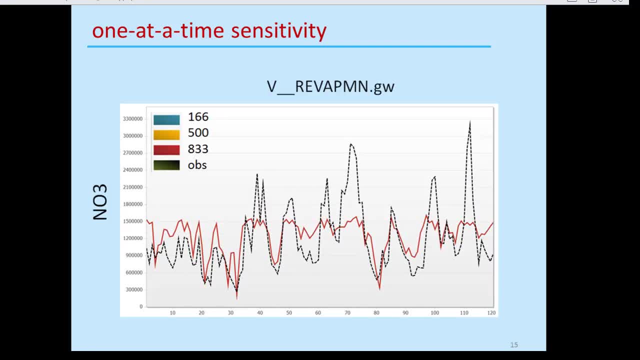 In another example. if I look at, for example, revap, minimum revap threshold, and I do three simulations similar as before, and I see only one curve here. so all three simulations coincide. So that means there is no. 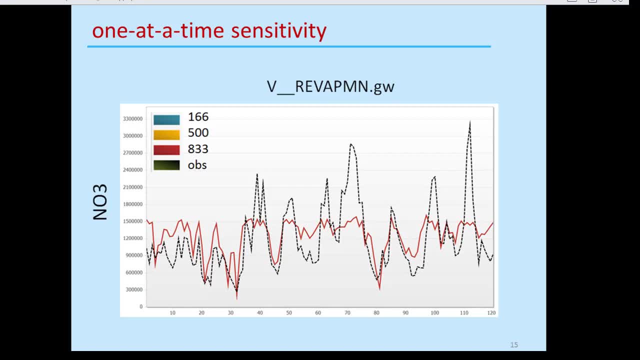 There is no sensitivity with respect to this parameter With respect to revap minimum. the model is not sensitive at all with respect to nitrate, So this is not sensitive. So there is no point. I mean you could include this in your calibration or not. 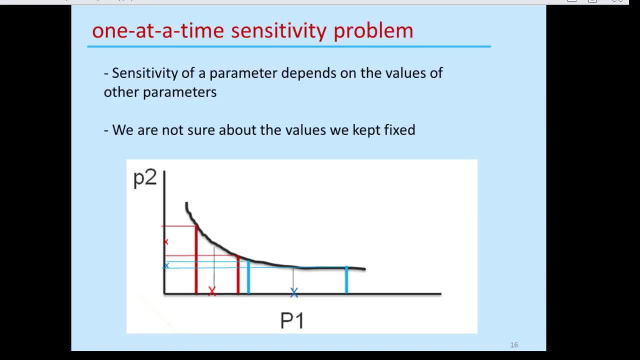 It doesn't make any difference. Now there is a problem with this whole concept of this one-at-a-time sensitivity analysis. It is sometimes useful, but it could also be misleading, in a sense that sensitivity of one parameter may depend on other parameters. 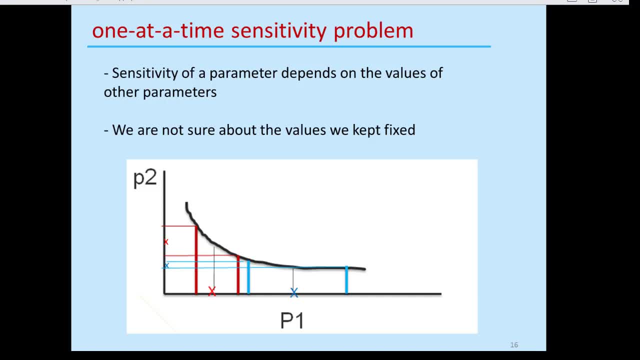 And here we have fixed the values of all other parameters to something that we don't know if they are correct or if they are not correct. Now to show: To show that the sensitivity of one parameter depends on the value of the other parameter which is fixed. 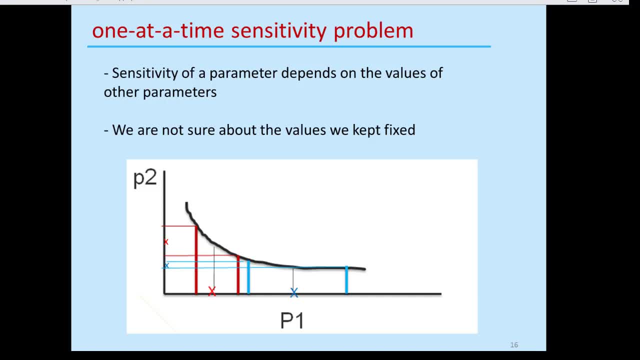 If I fix the value of my P2 parameter to this blue line here, point here, and then I look at my P1, I start changing my P1, right around this value, around this value. this curve here is the value of my objective. 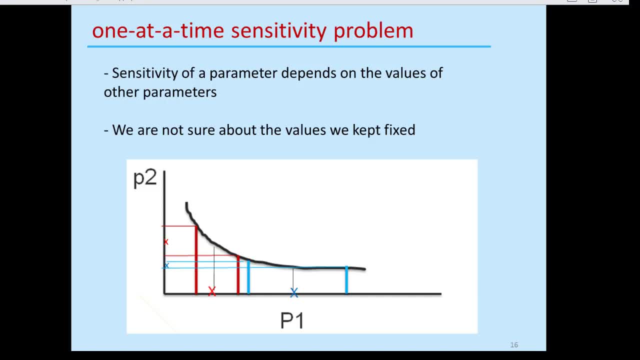 So this is my parameter 2,, parameter 1, and the objective function here. So I see there is no difference in the objective function. So if I happen to be in the flat part of the objective function with respect to a parameter, then changing parameter 1 doesn't show me any sensitivity. 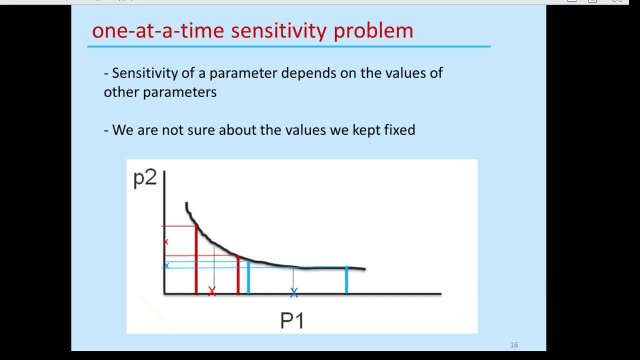 So I may conclude that P1 is not sensitive, Whereas if I had fixed my P2 value to this point here, which is a point- This is a point that I have a large change in the value of the objective function if I slightly move to the left or to the right. 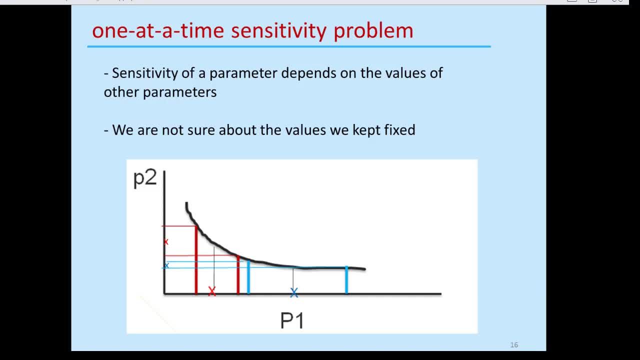 At this point, if I change P1 value within this range, I see a big sensitivity with respect to the parameter P1. So I may conclude that, yes, P1 is sensitive Here. I may conclude that P2, P1 is not sensitive, simply because of. 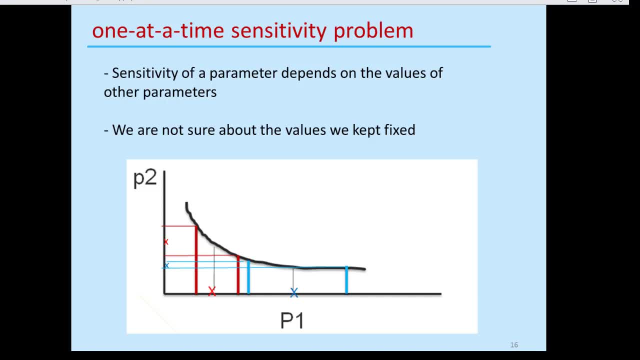 where the parameter P2 is fixed initially. So this is one problem with this approach is that we are fixing all parameters and we don't know whether they are at their true value or not, So we may be misled depending on the values of the other parameters that we have fixed. 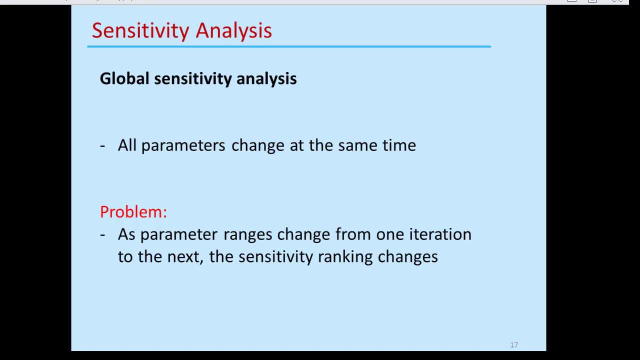 Now another approach is global sensitivity analysis. In the global sensitivity analysis, we are changing all the parameters at the same time. Now, the problem here is sort of similar to the one before- is that now we are dealing with ranges of parameters and the parameters are changing within a certain range. 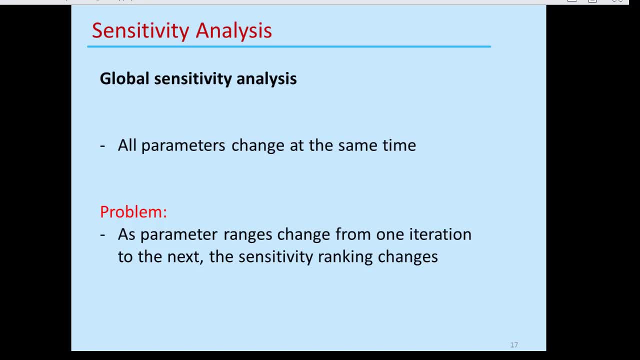 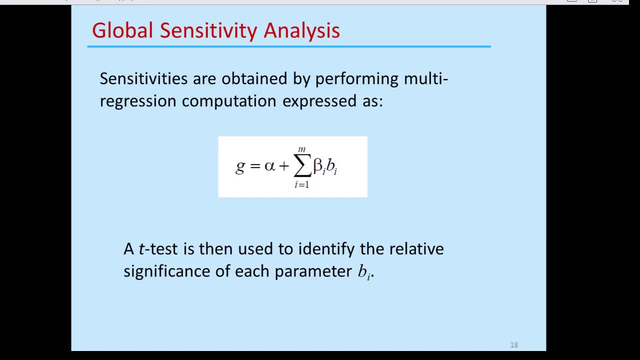 And now, if I change that range, I may get a different result. To calculate the global sensitivity analysis, we use a multiple regression computation such as this, where my objective function is a constant, plus this, my parameters times a certain coefficient, And then you perform the multiple regression and you calculate the t-test of this. 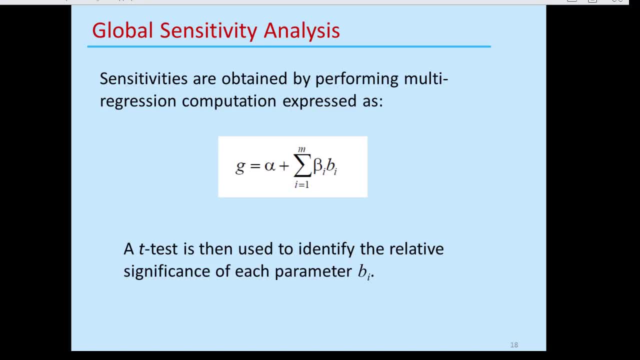 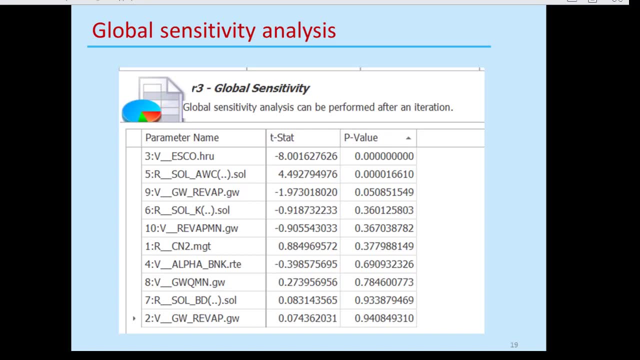 And then what we report at the end are the parameters and their t-test and the p-values, And you will get in SWAT cup something like this, which gives you the t-stat And the p-value of the parameters that you use. Now here we want to have a very small p-value and a very large t-value. 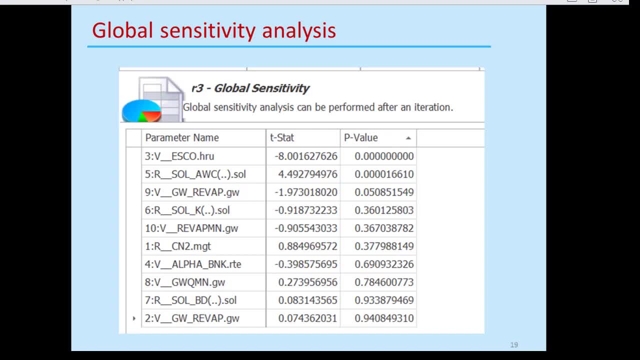 So the larger the absolute t-stat and the smaller the p-value. that is the most sensitive parameter. Sometimes you may have a large value- a large, I mean significant value- for t-stat, but the p-value may be very large, not small enough. 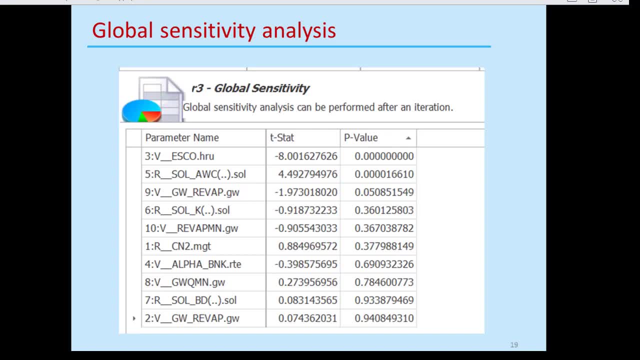 And that means that maybe the number of samples are too few and it's just by accident that this parameter has become sensitive as a large t-stat. But if it has a large t-stat and also a very small p-value, then it is a sensitive parameter. 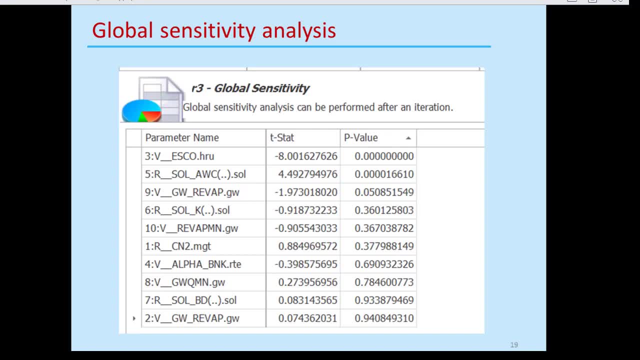 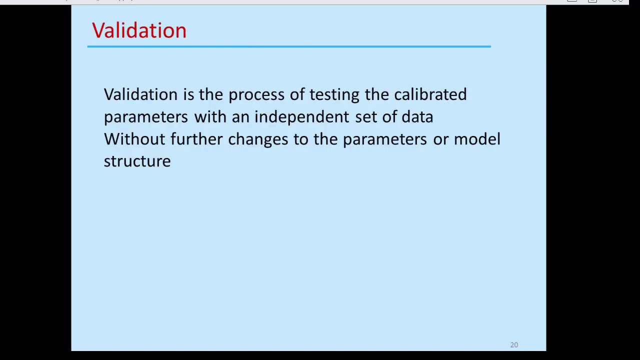 So, as I said, the problem is that in every iteration the ranking may change, So it's best to report this In the final iteration where you are sure of sort of the ranges. But that's the global sensitivity analysis. Now validation. 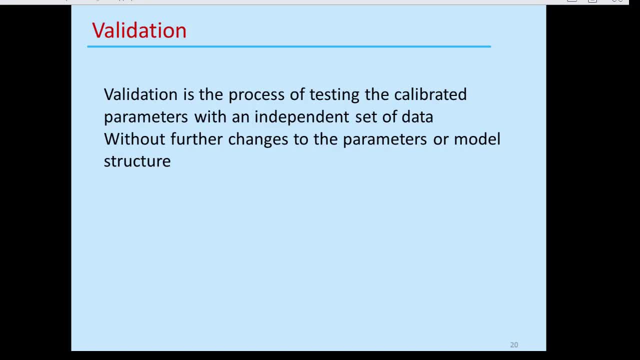 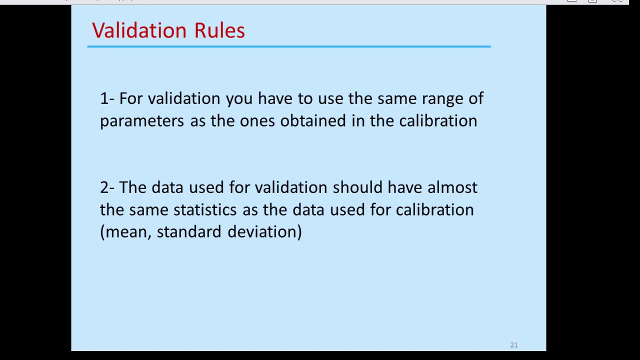 Validation is the process of testing the calibrated parameters with an independent set of data, without making any further changes to the parameters, And this is. There are two rules that should be followed when you're doing validation. The first rule is that you have to use the same parameter range and the same model, and 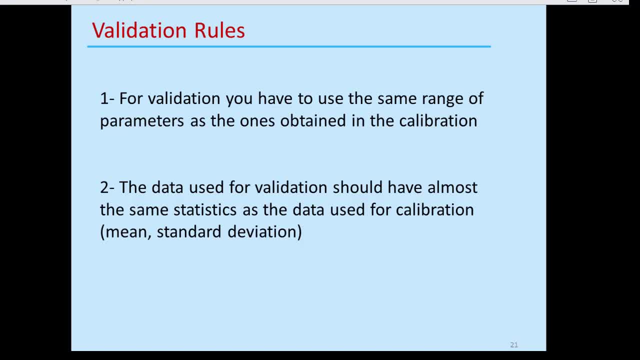 everything the same right? Because when you calibrate, you're conditioning your parameters on the calibration data set. So you have to make sure that this is not too conditioned on the calibration and it's also valid for a different data set. So you have to make sure that this is not too conditioned on the calibration and it's also valid for a different data set. 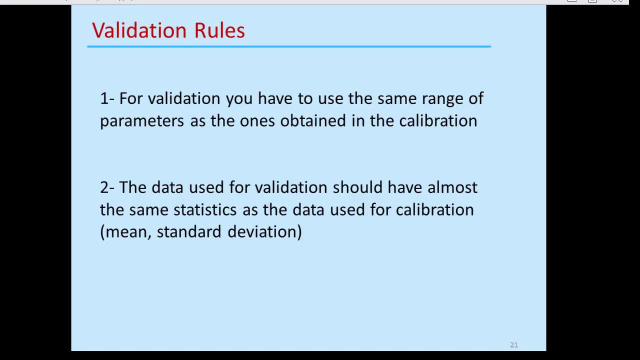 So that's why validation data sets should be different and independent- different from calibration data sets. And then you have to make sure that the data that you're using for calibration and for validation are more or less the same in terms of the mean and standard deviation of the variables that you are looking at. 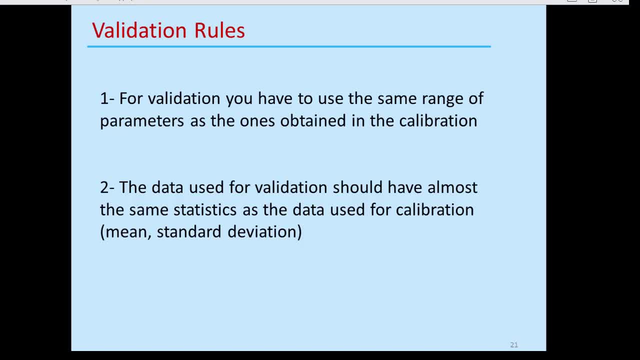 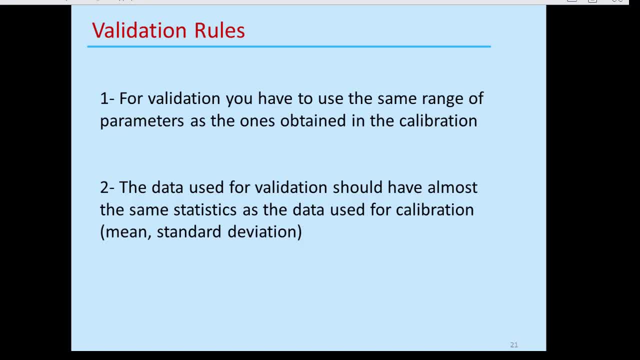 In other words, you should not calibrate your model for a number of wet years and then try to validate your model for a number of dry years, right? you should not calibrate your model for a number of wet years and then try to validate your model for a number of dry years, right? 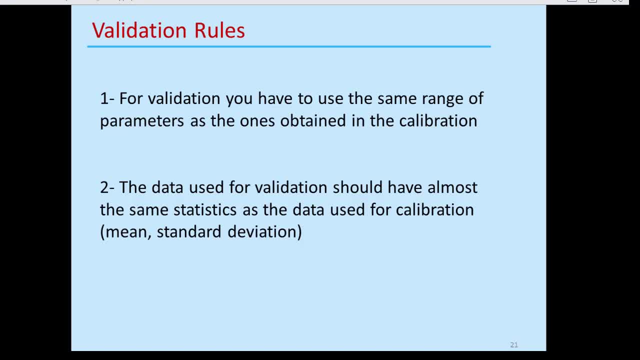 your calibration data should cover all kinds of climatic situation, so the two should have sort of similar statistics. and also this is wrong. i mean people ask me if they can use this for years of 2000 to 2017 for calibration, and 2012- 2017. 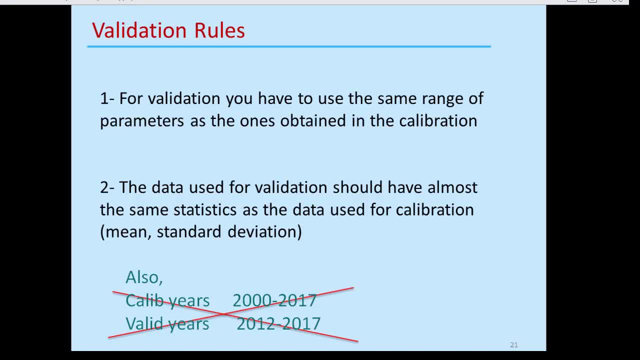 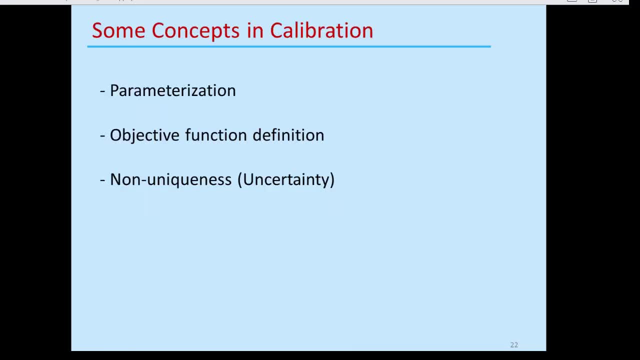 for validation. this is not correct. they should not overlap. they should be independent data set from different time periods. now let me cover some concept, important concepts in calibration, and these are parameterization, objective function definition and non-uniqueness or uncertainty. now parameterization: there are two issues in parameterization, or two. 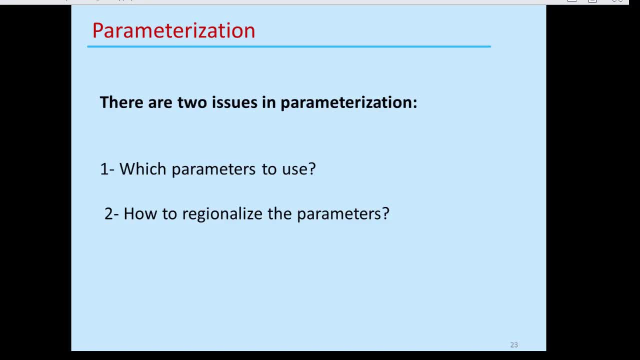 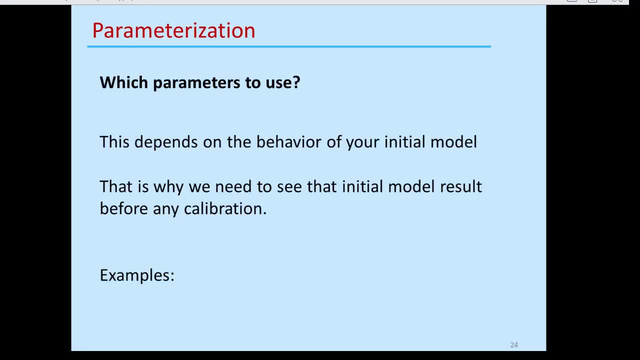 questions. one is which parameters to use and the other one is how to regionalize these parameters. so let me explain, okay, which parameters to use. this depends on the behavior of your initial model- and let me tell you the parameters you choose and you can see. they are very simple, right? i see often people send me 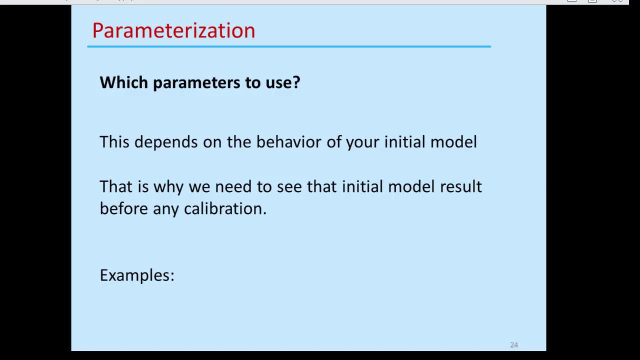 questions and so on, and i look at their parameter file, the part in file, and they are like everything is in there, like 20 parameters, whatever they could find, they put in there and try to make a run and hope to get something out of that. that is not the way. 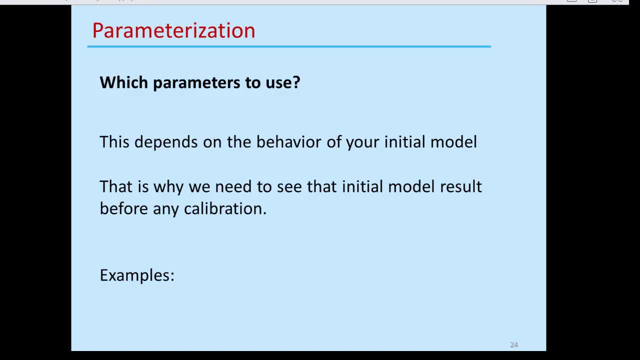 you should do it- the parameters that you choose of your, your initial model. that is why we need to see that initial run. i emphasize that: what is the initial run of your model? let's see how that looks first before we go any further. now i give you some examples. if your 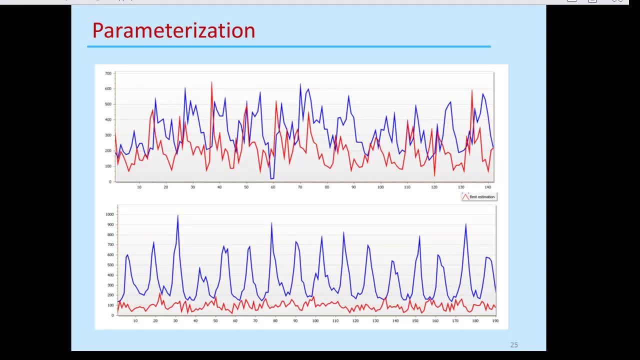 initial model run looks something like these two, then there is no point in calibrating this model. i mean, there is clearly something is missing, something is wrong here. either you are at the downstream of a dam or something, or your precipitation data is completely wrong, because there is a complete mismatch. 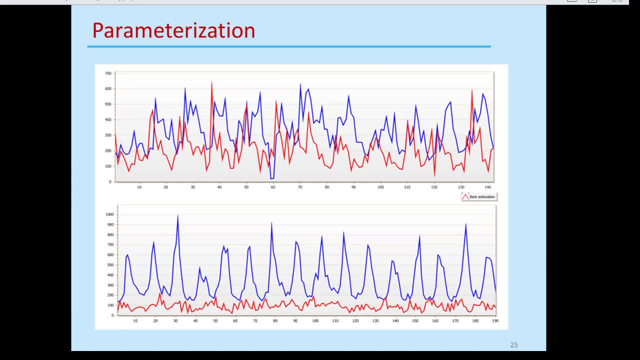 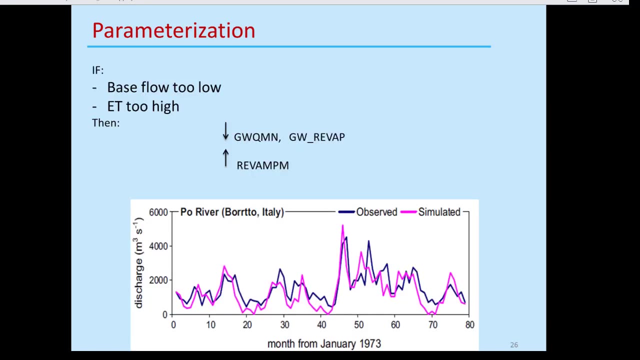 between the two: the simulation and the observation. so in this case i would just go back to the model and see, re-examine my model and the processes and the data and all of that. now, if you get a situation like this that you have systematically lower base flow, so if your base flow is too low, 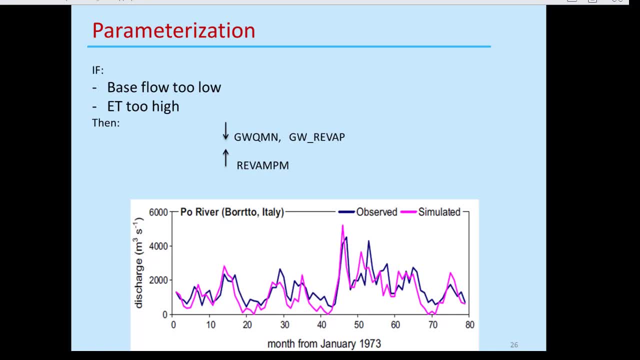 and your et is too high, then what you need to do is to set these parameters. you need to lower these two parameters and you need to increase, rev up the minimum, rev up this parameter. so you need to decrease these and you need to increase that in order to get a higher base flow. 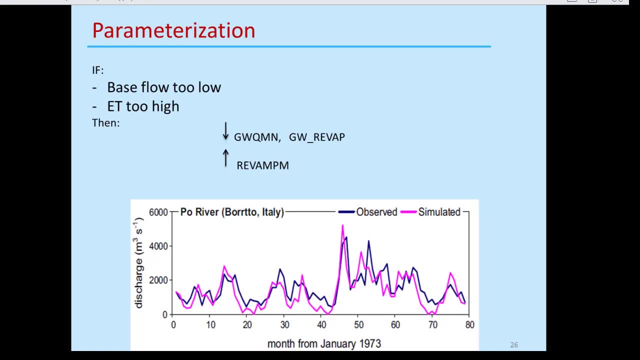 so, from the parameter point of view, these are the parameters that you have to change now. it may be that this lower base flow is because there is a groundwater flow. there is an input into your model that you are not aware of. there may be a point sources that you are not aware of, but from parameter point of view, these 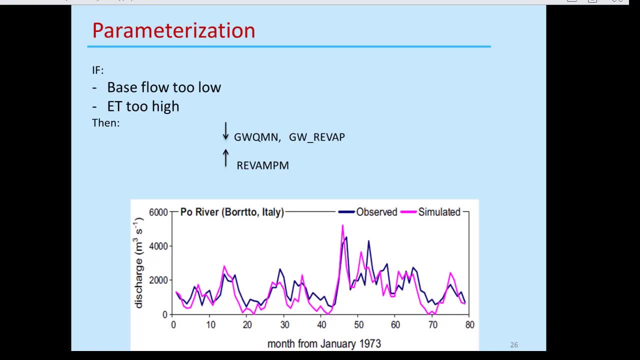 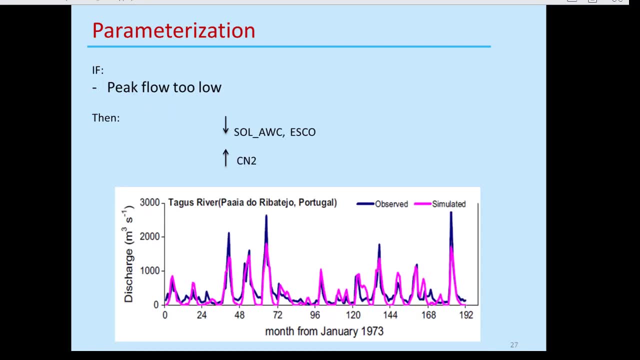 are the parameters, but from process point of view you have to look at the what is coming into your river from other sources of water into your river now, if you have a situation like this where your peaks are systematically low, so if your peaks are too low, then you need to decrease. 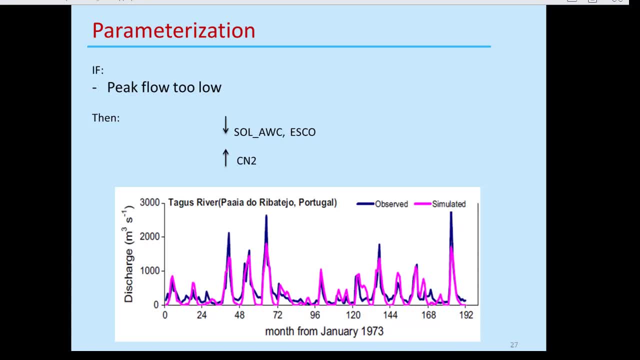 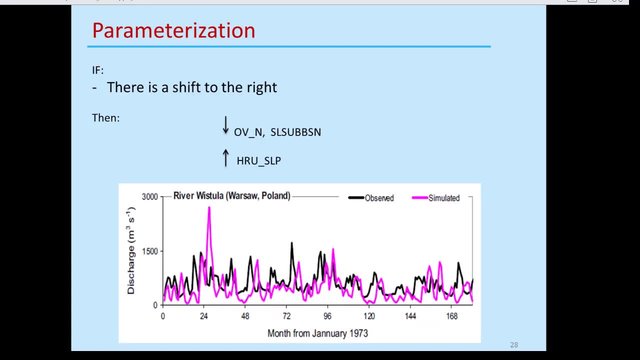 these two parameters and you need to increase cn2 if you have a shift. if there is a shift, a systematic shift, always your peaks of your simulation are to the right or to the right shifted to the right, then you need to decrease these two parameters and increase this parameter. 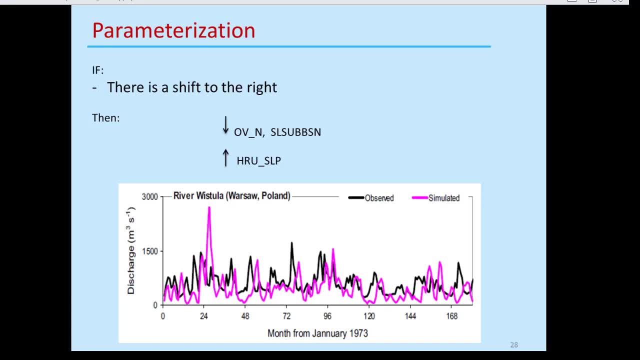 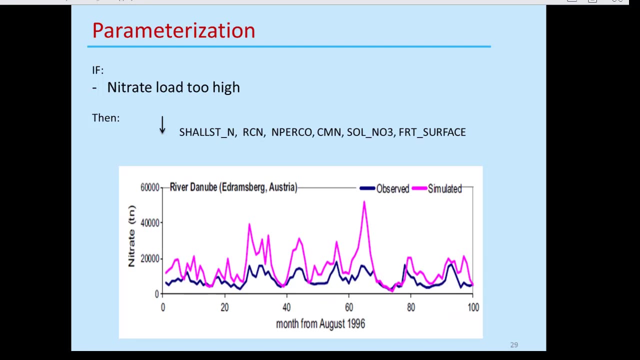 now, if it's the opposite of this, if it's too too fast the peaks, then you need to do the opposite, that you need to increase this and decrease those. finally, if your nitrate- if you're looking at nitrate and you have a situation like this where your nitrate load is too high, then 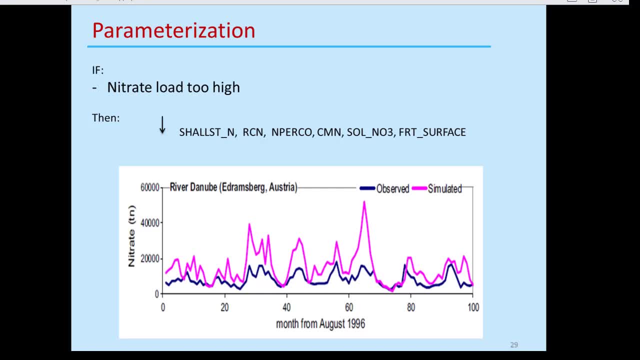 you need to decrease one or more of these parameters. so the moral of the story here is that you have to look at your model behavior and then choose the parameters to achieve a certain change in your model. so don't just randomly pick 20 parameters and, you know, put everything in a pot and try to get something out of that you. 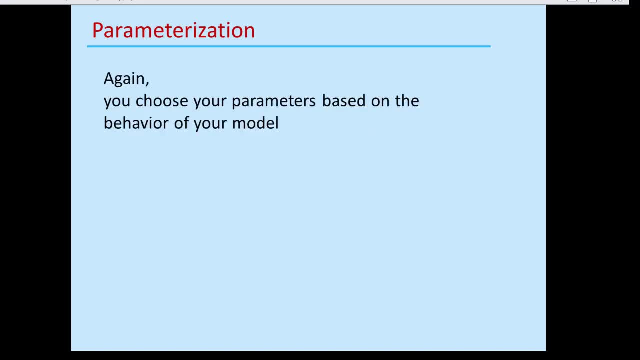 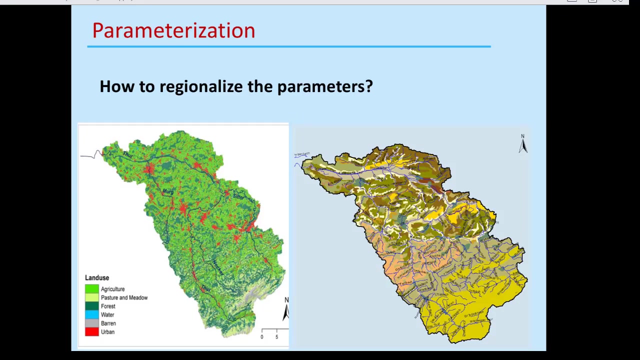 have to look at your initial model run. so again, you choose your parameters based on the behavior of your model. now, for more detail on this, you can look at this European paper that we have published in in this journal. now. the other was the regionalization of the parameter, and what does that mean this? 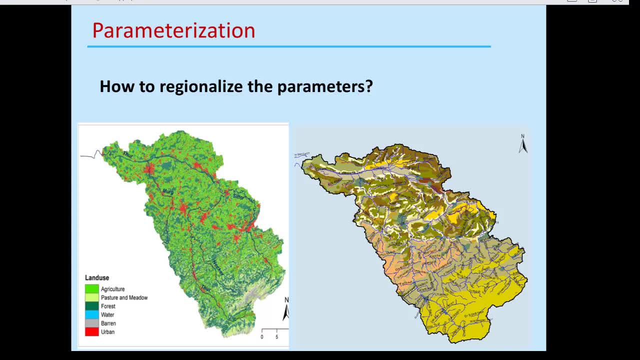 is the soil map. on the right is a soil map of the tool watershed and this is the land-use map. now, in the soil map, you often have the same soil unit appearing in different places. it's the same soil unit, so this soil unit has the same parameter value everywhere, right? but 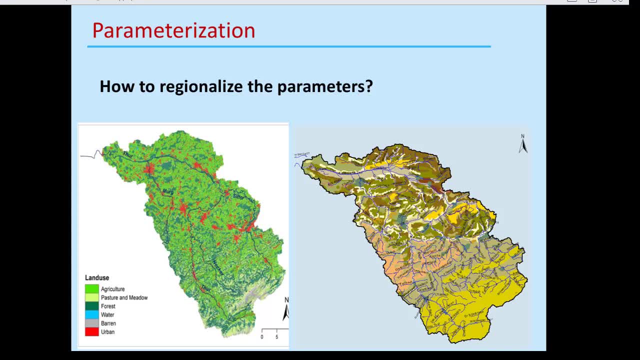 here you may be on the forest, here you may be under agriculture, here it may be pasture and so on. and when the soils appear under different land uses, the parameters of course change. the soil surveyors don't look at the land, I mean they don't look at the hydrology to set soil parameters. so 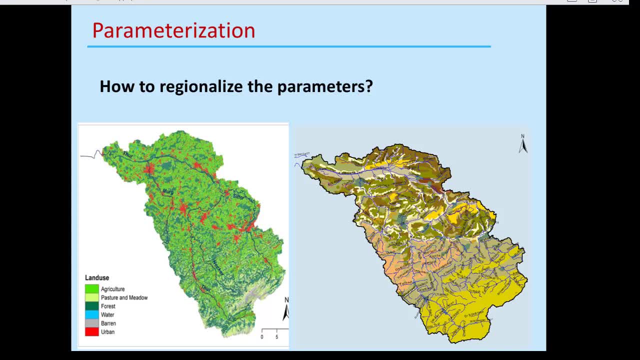 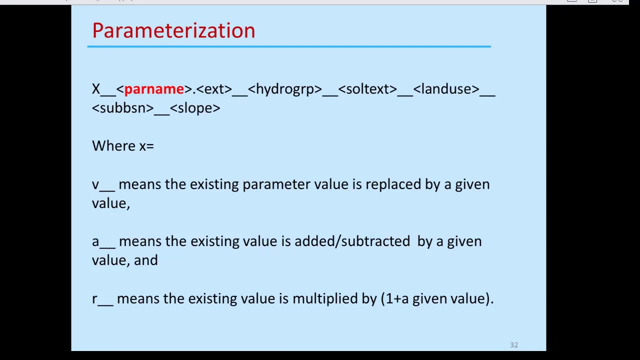 those soil units may have nothing to do with the hydrologic behavior of those soils. so you want to be able to change the same soil unit, its hydraulic conductivity value, under forest or under pasture or in a mountain or so on. so for this purpose, to regionalize those parameters, we have devised a system such 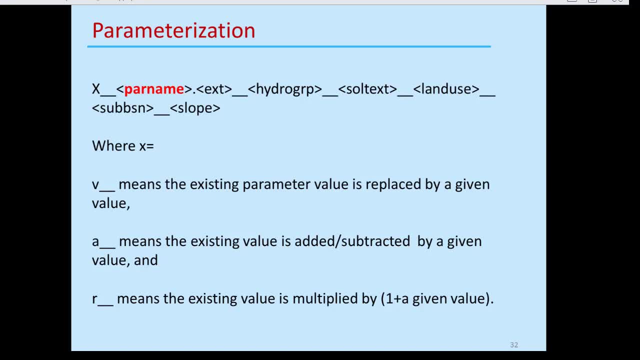 as this, that the parameter can change its. you can change the value of a parameter with respect to its hydrologic group, soil texture, land use, sub basin number and slope, or any combination of these. so this is calibrating a parameter at the HRU level, in this example X. here it means if it takes the value of V, if I 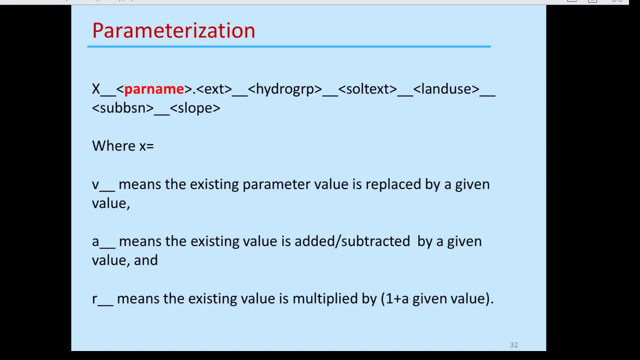 put V here, it means that you are changing the existing value with another value. if I put a, that means you are adding to the existing value or subtracting a given value, and if I write our here, it means that it's a relative change, that you are multiplying the number already, the- the value that exists- by 1 plus a. 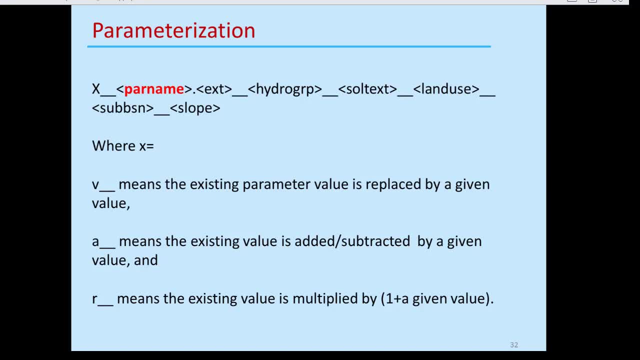 certain given value. so the value that multiplied by a certain value. there are some parameters in SWAT that are spatial, that means they change from place to place, such as soil parameters, CN2 and so on. and there are some parameters that are not spatial, such as groundwater parameters, that SWAT uses. this the same, the same, unless you have information of 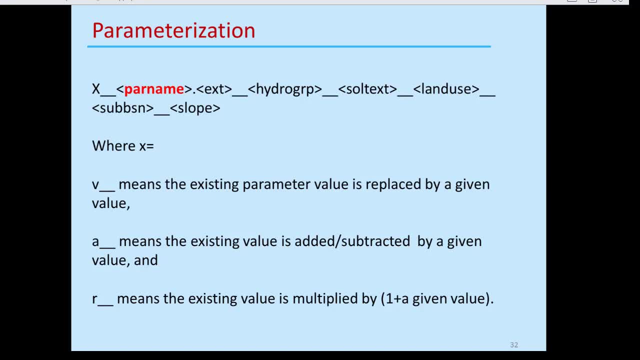 course you change these parameters, but they are not spatial and there are some parameters in the basin that is defined at the basin level. so those you can change one value for another value. but the parameters that are spatial, you cannot just set one value everywhere. so you have to be very careful and you have 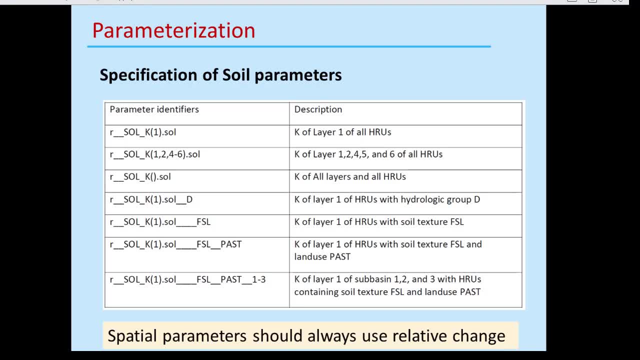 to make those a relative change. now here are some examples. you can also see these in the manual, so I don't want to spend too much time here. but the first thing you need to do is you can change the soil hydraulic conductivity of the first layer in a relative change. that's what this means. so that's the 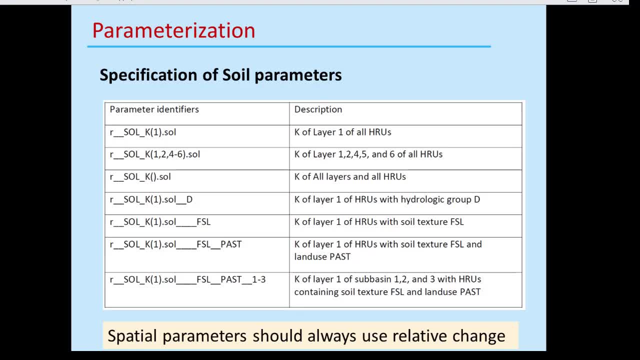 syntax of how you would express this, how you would specify. so here the relative change of soil hydraulic conductivity for layer 1, layer 2 and layer 4 to 6. so that's the syntax, how you would write that if you don't write any thing in the bracket, things that are meant can take many values, like 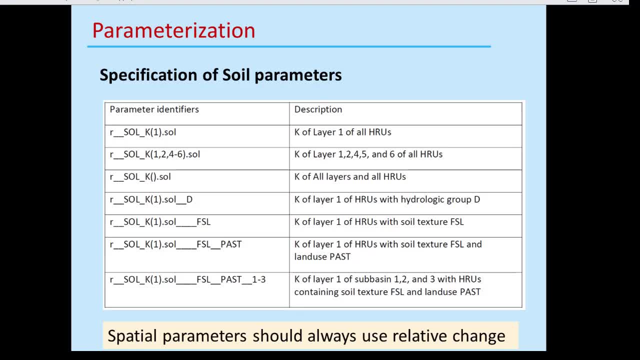 hydraulic conductivity can have 10 layers. so those parameters have a bracket and you have to specify the layer. if you don't write a number here, that means all the layers. if I write relative change of soil hydraulic conductivity for layer 1, if soil hydrologic unit is D, if soil texture is: 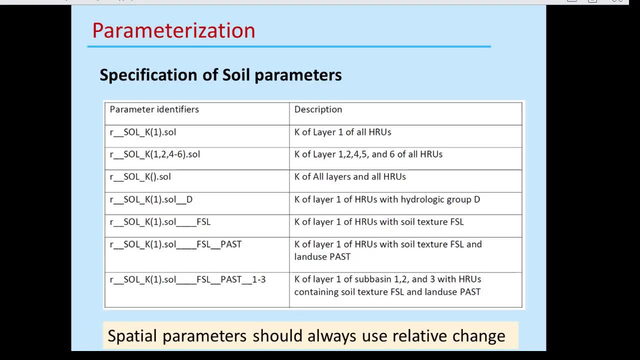 fine sandy loam. if soil texture is fine sandy loam and it's under pasture, if it's fine sandy loam under pasture and it's in sub basin number 1, 2 and 1, 2, 3, then you have quite a bit of flexibility in really setting parameter values and you can use. 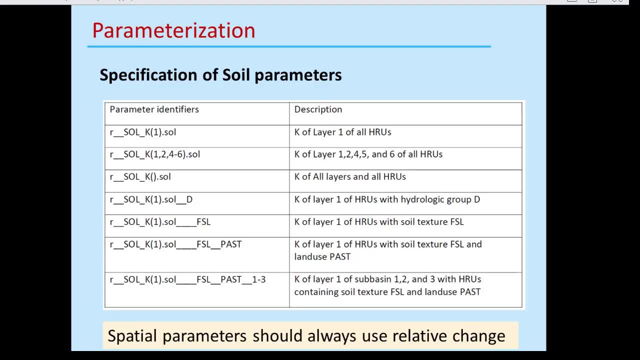 this flexibility. the thing is that if you go too extreme in this direction, you will end up with too many parameters, and if you go to extreme in the other direction, you can generalize. you can lump everything and lose the variability in your watershed. so you have to be careful how you parameterize. 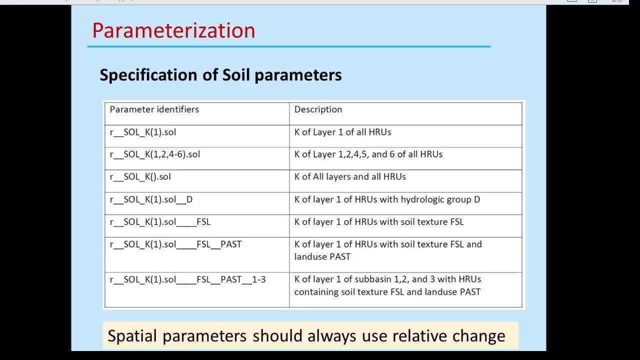 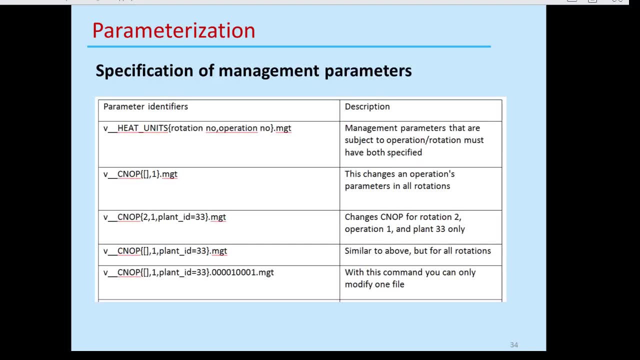 here, but it's important to note that the spatial parameters should always be relative change in the spatial parameters. you can do the same parameter change in file, for example management files. management files are specified by rotation number and operation number, so you can change the CN value for all. 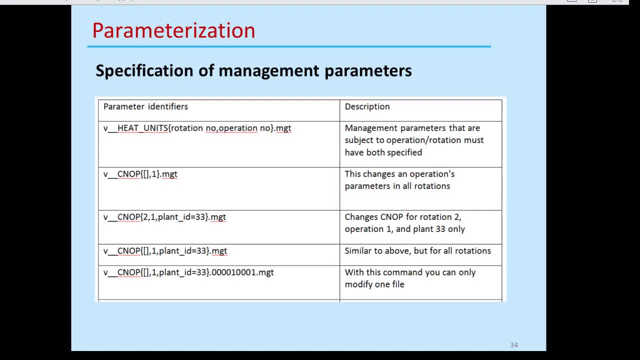 rotations operation number one or rotation number two, operation number one for plant number 33, or of all rotations operation number one, plant number, ID number 33 and so on, or you can specify a certain file and just change the values in that certain file. again, you have a lot of flexibility in. 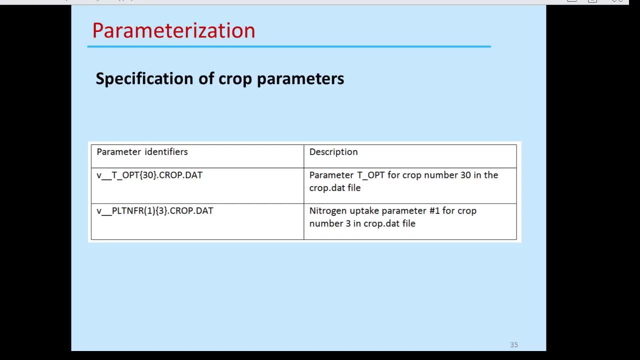 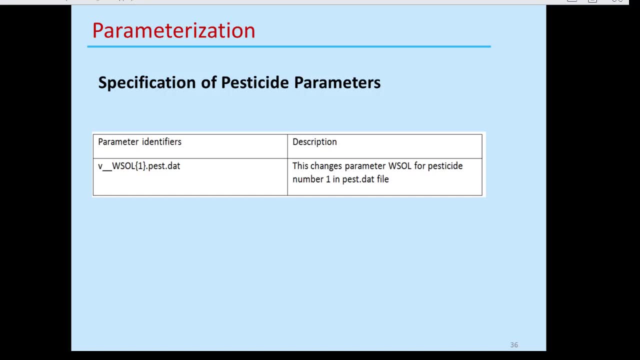 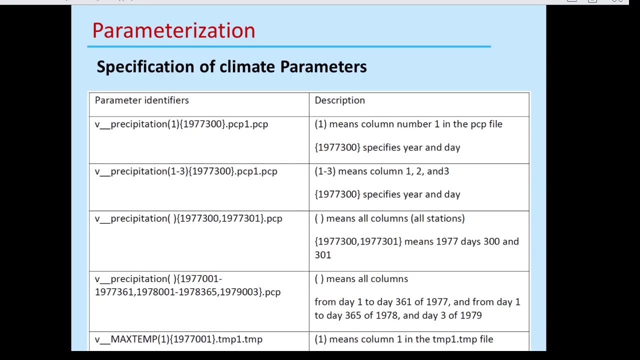 changing management parameters. similarly with crop parameters in the in the crop dot that file, similarly with pesticide parameters in the pesticide data file, and so on and so forth. and finally, the most important one, is personalization. I have added this because sometimes you have a lot of missing value and you use 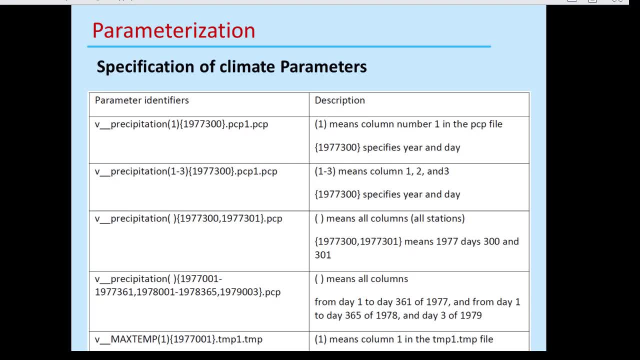 W gen and SWAT generates numbers for those missing values and those generated numbers could be quite wrong. so you should be able to to fit some of those numbers. but you have to use this option very carefully, because if you fit rainfall, then you can fit any kind of discharge, so you should not. 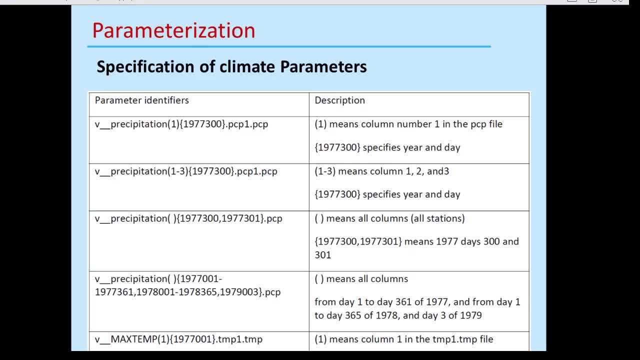 use this for fitting your discharge. this is only to set some values that you know is different from the value that are reported, and here again you have a lot of flexibility to change the value of rainfall for one day for one station, or for a number of station and one day, or for all stations and some days, and 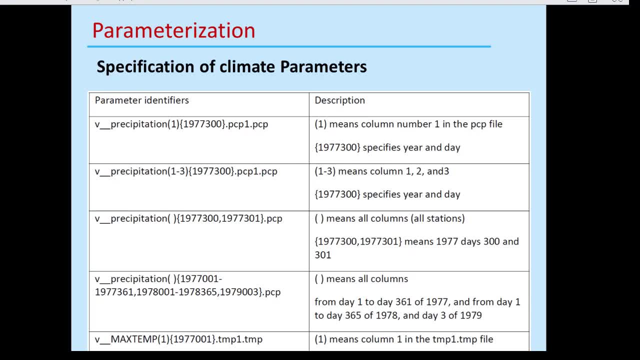 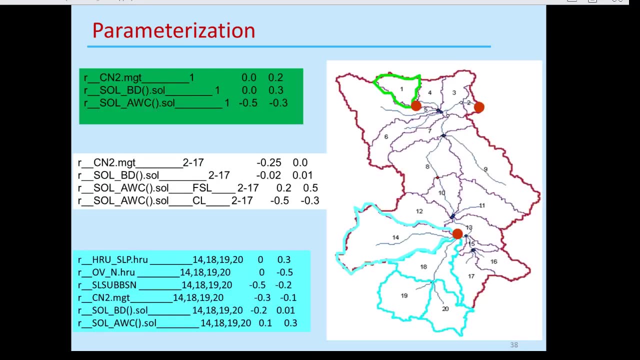 you can change for the whole year. thedio愛, multiply the whole year by certain numbers and so on. A lot of flexibility also here to change rainfall. So that's what we mean by parameterization here. Another aspect of parameterization is that if you look at this example and you have three outlets, 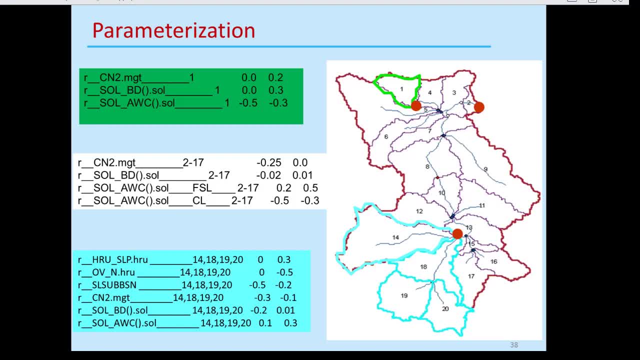 this outlet is fed by this sub-basin right, So changing values here doesn't affect that sub-basin at all. So if I want to fit the discharge here, I can only change the parameters of sub-basin number one. So here I look at the behavior of sub-basin number one. 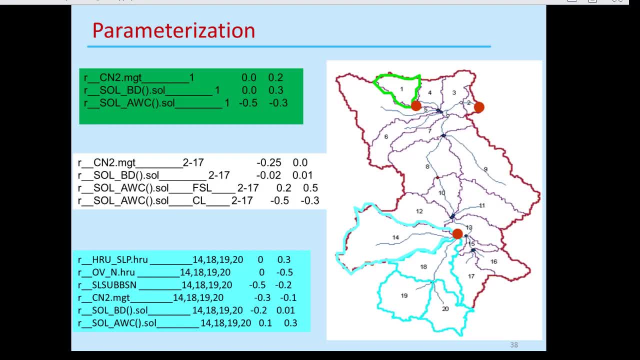 and I choose the parameters according to model behavior here For this outlet. these sub-basins are important Or are affecting coming into this outlet, So I need to fit this. I need to change the parameters of these sub-basins only. 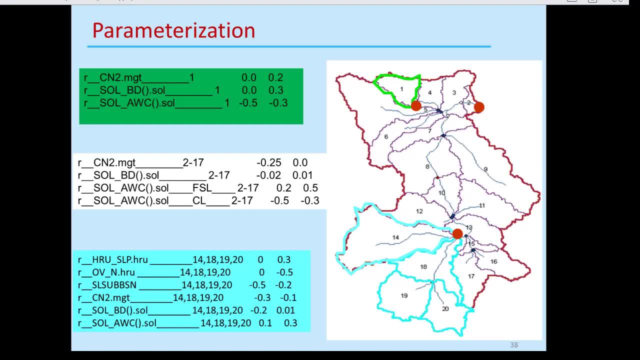 And again I look at the behavior of model here and I choose parameters that give me the best fit to the model here. This is the outlet of the whole watershed And after I have done this, parameterized this and this, then the rest of this sub-basin. 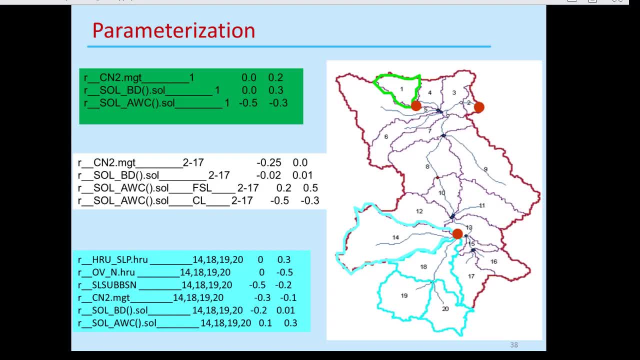 these sub-basins are the ones that are contributing to this watershed, So for those, I can again set the parameters of these so that I can achieve the best situation here. So this is a very important parameterization and you really need to follow this in your model to get the best result. 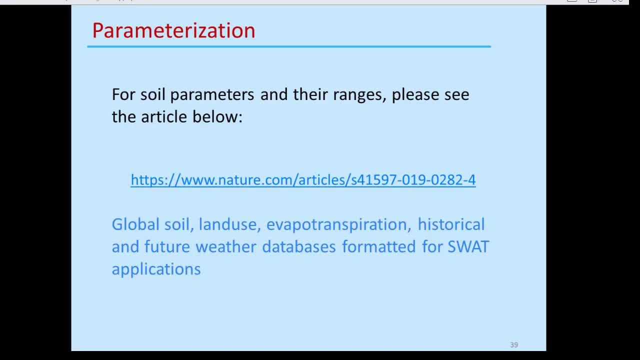 Now you can look, read more about this and you can also see the data in this file here And this file here. this report here has values of soil parameters for different soil texture. So if you have a clay soil, the range that you can use for its soil parameters is different. 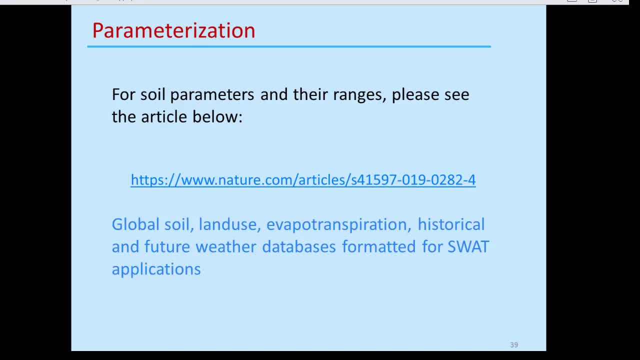 if you have a loamy soil. So based on the texture, you can choose a better value for the ranges for the conductivity bulk density and so on and so forth. So I highly recommend that you have a look at this article here. 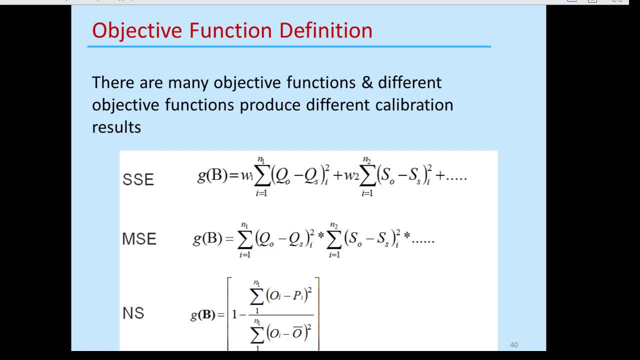 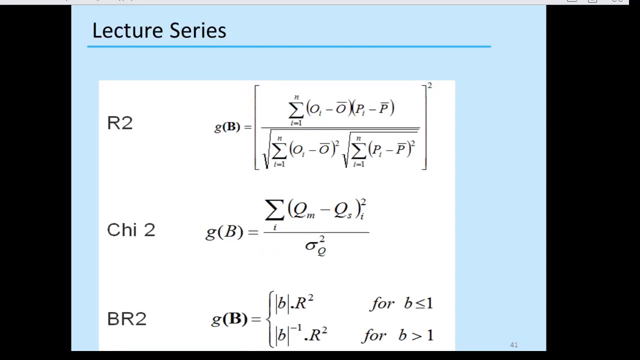 Next is objective function. Objective function: there are many, many different objective functions in the literature and we have 11 of them in the SWAT programs. Now, here you see the sum of square error. Here you see the square errors multiplied. Nash-Sotcliffe: r. squared. chi squared. br- squared. 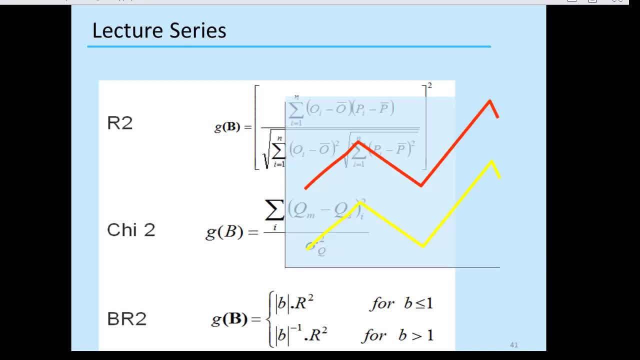 a lot of different objective functions. We don't normally like to use r squared because, as you see, these two signals here have r squared of 1, whereas the magnitude is very different. So if you want to use r squared, the best would be to use br squared. 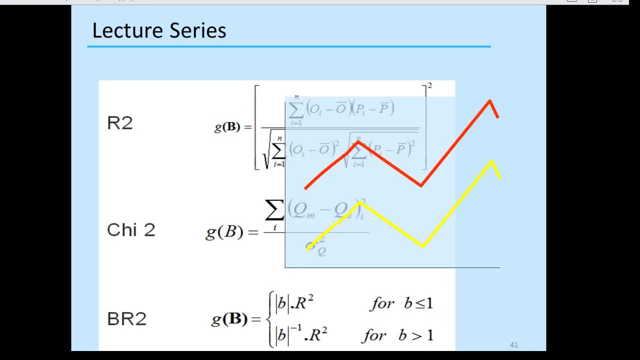 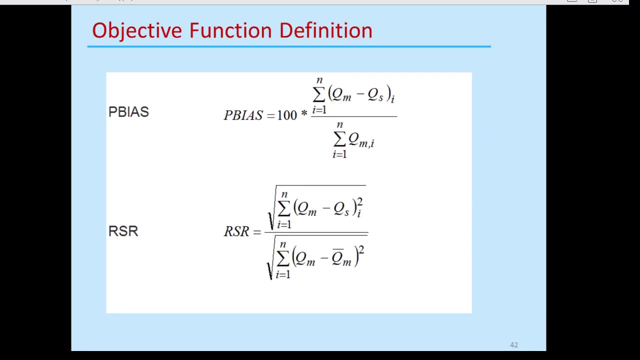 where you multiply r squared by the regression constant between these two. So you sort of take into account the magnitude as well as the linearity. So br squared would be a much better option to r squared. And then you have p-bias and rsi. 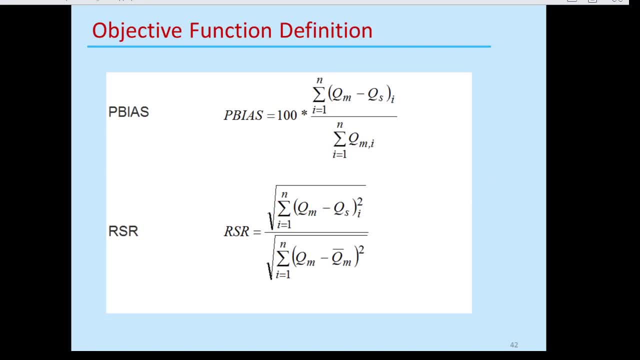 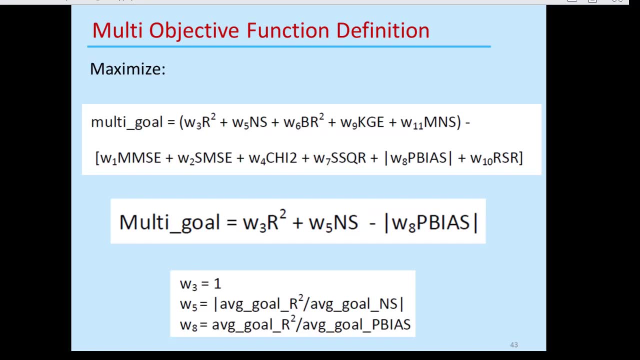 I have added these over the years as people asked me, And recently in the SWAT Cup Premium. we have added multi-r. We have added multi-r objective functions And what it does is uses these 11 objective functions and tries to maximize such a function. 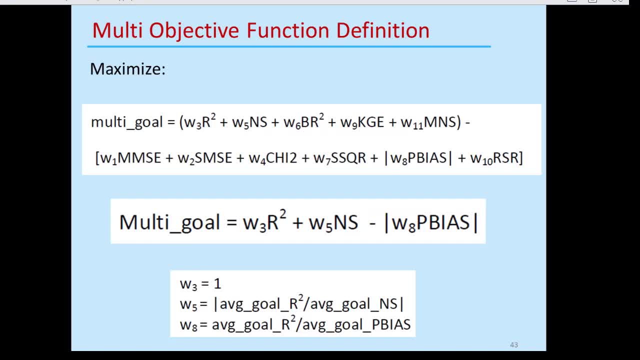 Now you can use this to build your own objective function, for example, using r squared, Nash-Sotcliffe and p-bias and with the weights And the weights we calculate, such as this in the SWAT Cup. Now, if you can build, 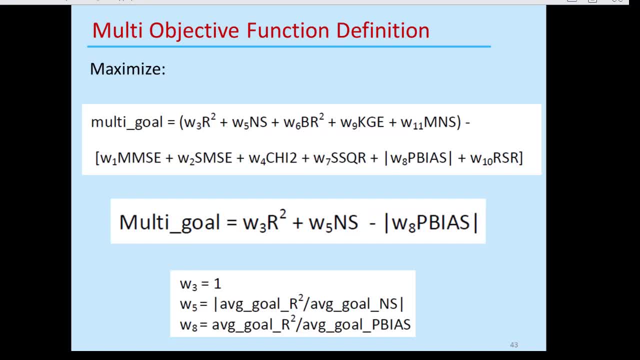 you can set other weights to zero. That means they are not considered. So you can really build your own objective function and see its performance. That's very important. It makes your result at the end independent of objective function. Right now the results. 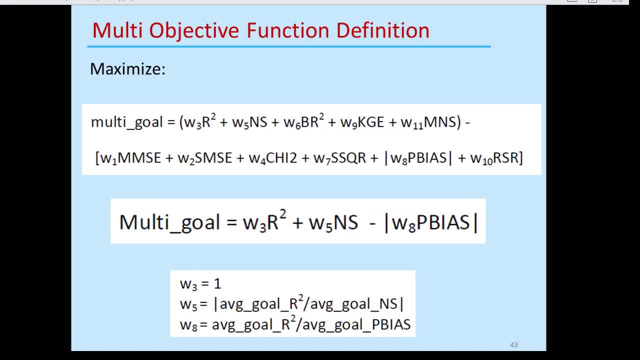 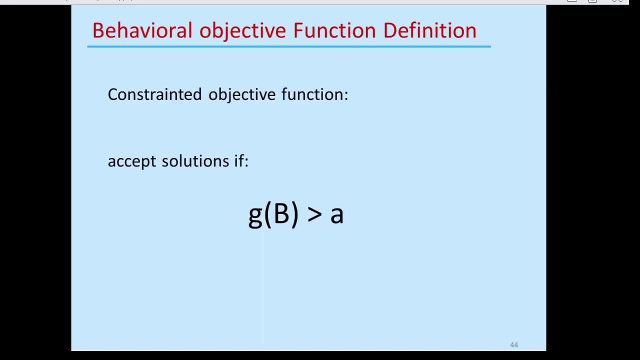 if I use r squared, then my calibration result is conditioned on the r squared, So it's a conditional calibration result, Whereas if I use many objective functions, then I can obtain an unconditional calibration result with respect to objective function. And then you have the behavioral objective function. 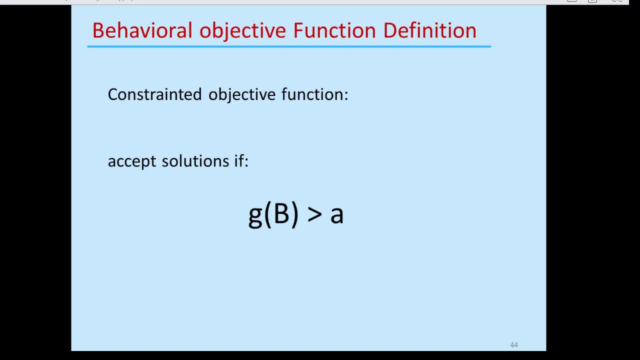 which is also- it's now included in the Premium version- where you can constrain your objective function. For example, if you have your objective function is Nash-Sotcliffe, you can say: I only want to keep the simulations where the Nash-Sotcliffe value 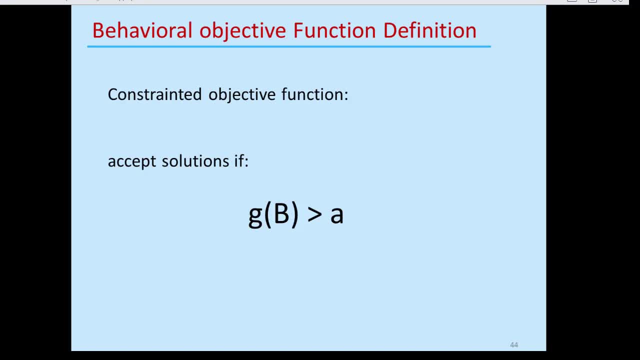 is larger than 0.7.. In that case if you do a thousand simulation, maybe 300 of those have objective function greater than 0.7. So you can only work with those 300. So you know that all the results. 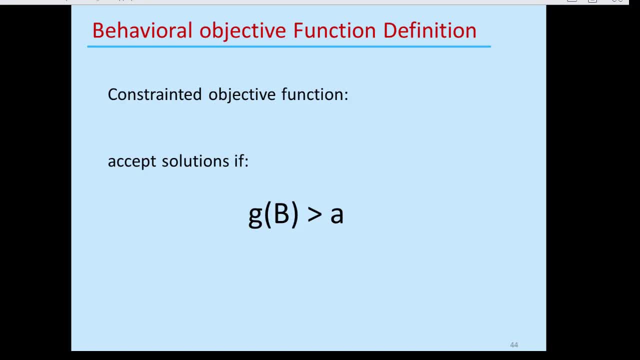 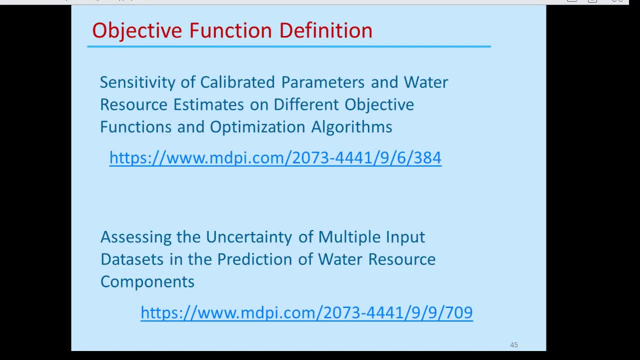 from your calibration are better than 0.7.. So it's also quite interesting to see how that performs. Now I would recommend you read more about the objective function and its sensitivity to the parameters that you obtain in these two articles here. 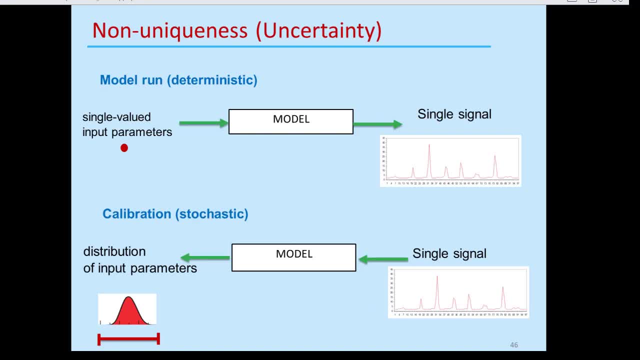 Now let me go back to this graph again about non-uniqueness and uncertainty. Now a model run is always deterministic. as I showed here, Calibration is always stochastic. That means at the end you have a range of values. Always you have a range of values. 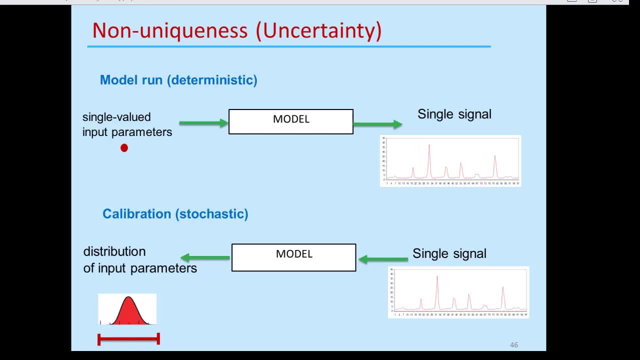 that you have to carry in your further analysis. So again, don't write me that you. how do I put the best parameters into the ARC-SWAT model or into the SWAT model? This is really it's not meaningful at all. 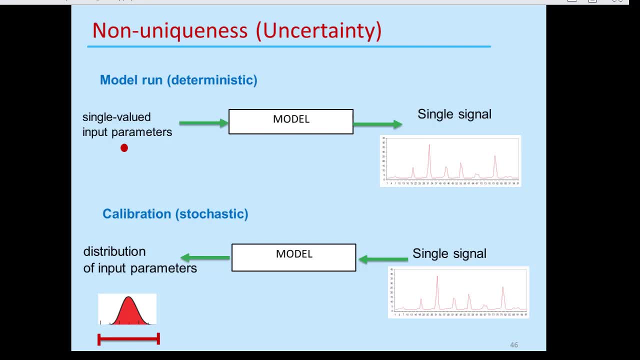 this question. There is no best parameter. You have a range for a parameter and then that's the range you have to carry in your further analysis. So forget about the best parameter and how you put the best parameter into the model, Although you can do that very simply. 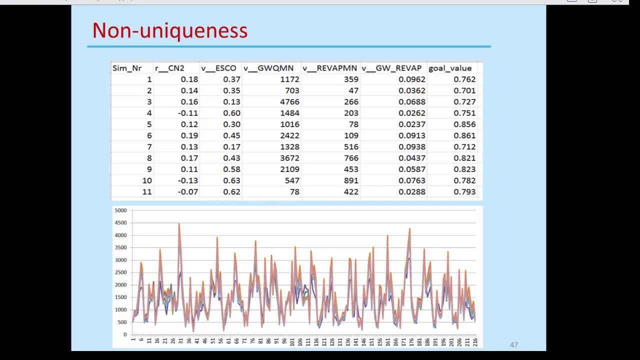 anyhow, Again with the question of non-uniqueness. here you see, we have many, many simulations and many parameter sets, which are all good simulations to my model, So I need to carry these everywhere in my further analysis of the model. 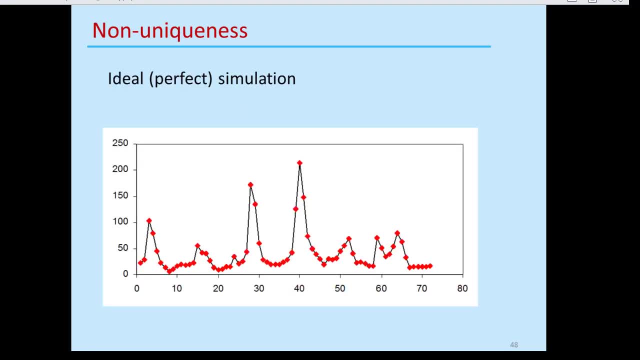 Now, an ideal situation is something like this: This is a perfect, non-unique, perfect situation, very unique, I mean. you don't have any non-uniqueness, You don't have any non-uniqueness, You have a perfect situation. 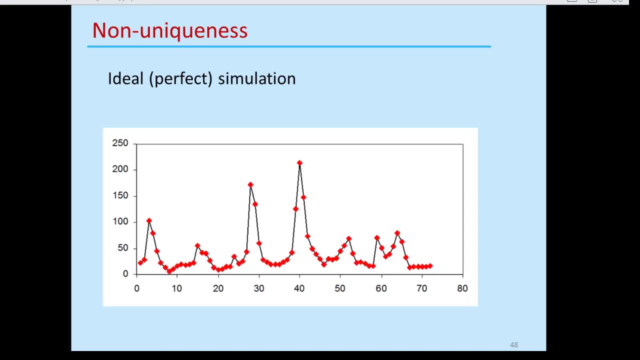 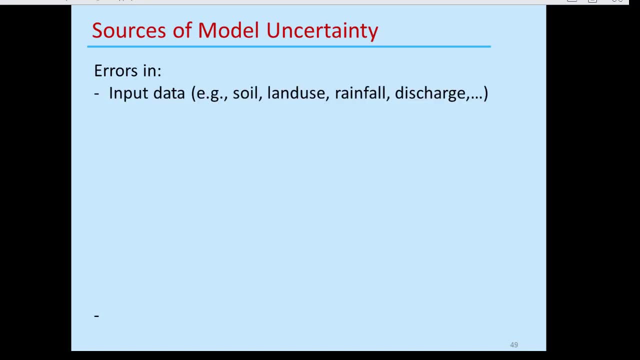 But we will never have this in practice. The reason is that, because of all the errors in the model, you have errors in input data, in the land use, soil, rainfall. even the discharge that you use to calibrate your model has a lot of errors in it. 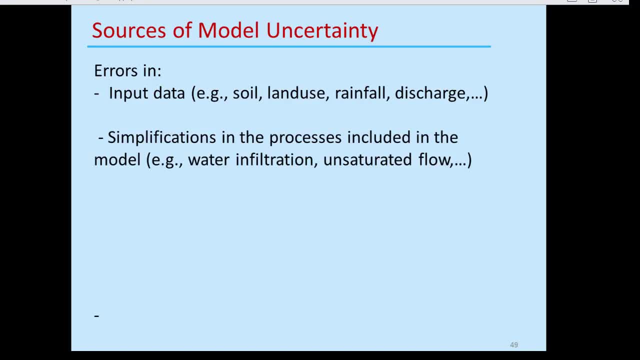 You have a lot of simplification in the processes that are included in the model, such as water infiltration through CN2 or unsaturated flow through these bucket concepts. These are very simplified processes. Then you have missing processes that are completely missing from the model. 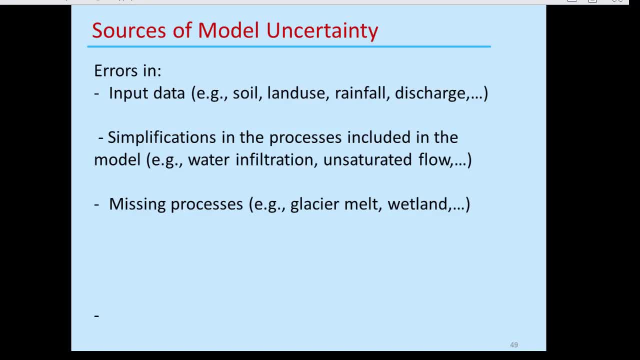 such as glacier melt, wetland and many other things. Then you have unknown model parameters such as CN2, soil, hydraulic conductivity. I mean, you haven't measured these for your watershed lab yet, So these are all unknown parameters. And finally, you have the uncertainty. 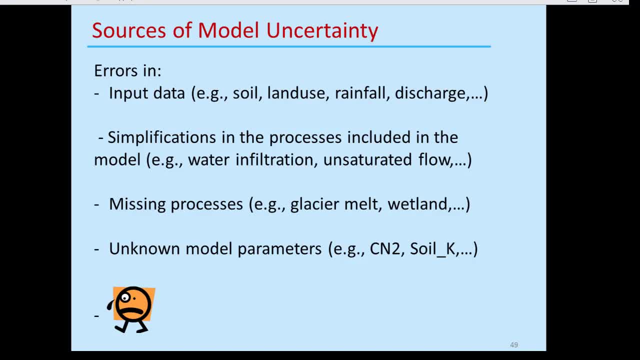 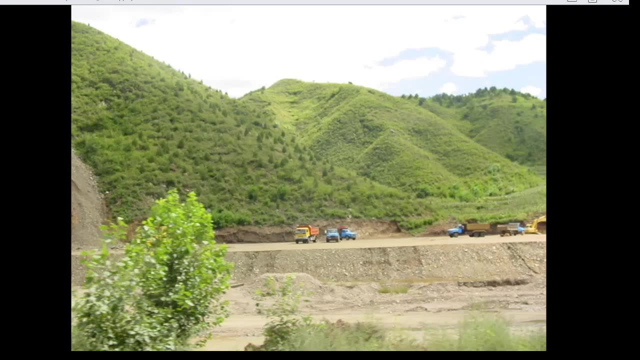 associated with the modeler. So you have a modeler who doesn't know what to do and it's not experienced, and he's just trying. So, given all these sources of uncertainty, you should not expect to have a perfect model, a calibrated model, at the end. 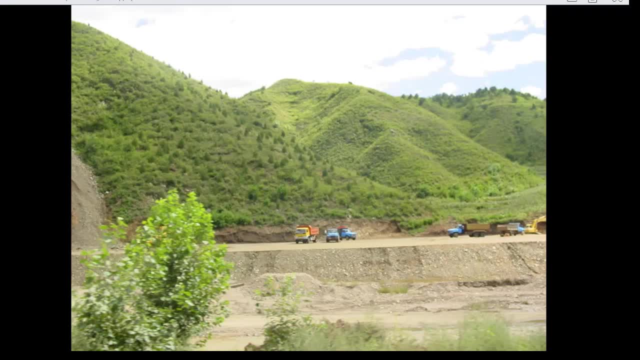 And some of the calibrations- that involves sediment nitrate, phosphate and so on- are really much, much more difficult because of the things that happen in the watershed. I leave you with this example that we had a project to model sediment in a Chinese watershed, the Haihe River Basin. 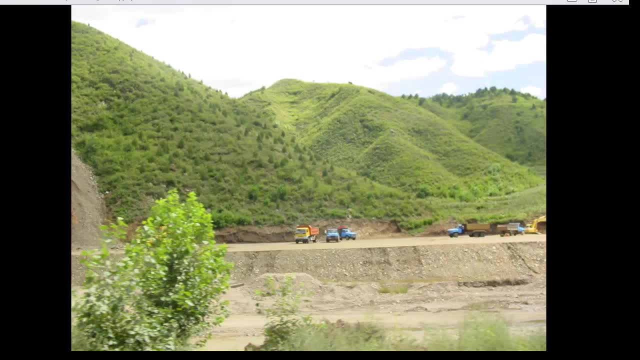 and we really couldn't get anywhere close to the reported observations. So we went to China and went up and down this watershed and I realized a lot of things going on in this watershed, such as road building. Here they cut the mountain to build the road. 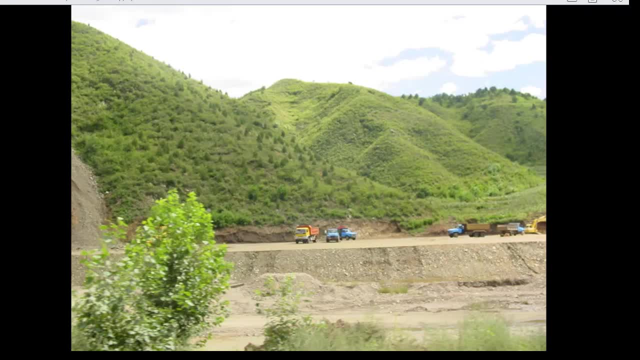 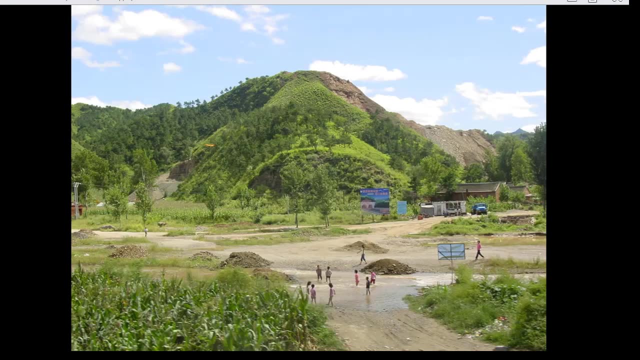 They take the material and dump it in the riverbed. And you have here, for example, this one example. They dump all these truckloads of material in the river. At the next rainfall, we'd wash away all the fine material, leaving behind pebbles and cobbles. 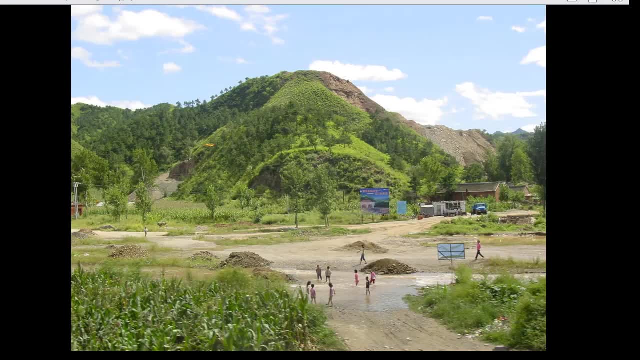 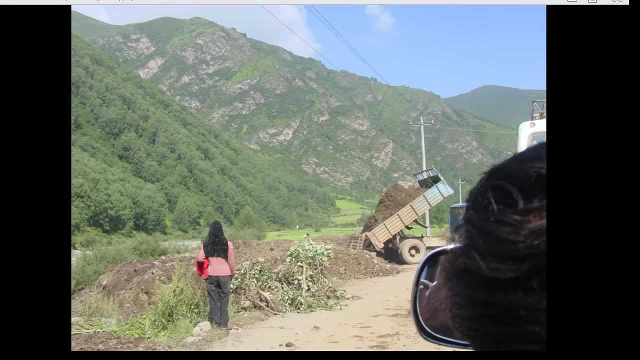 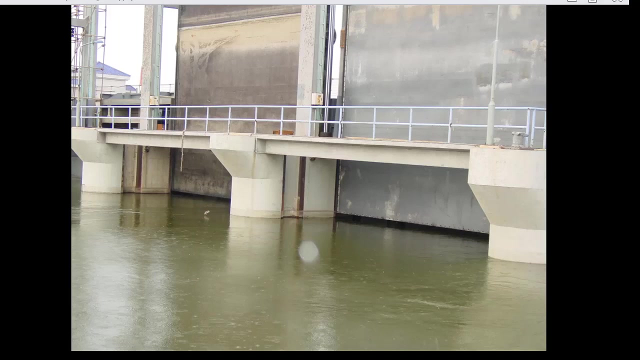 that they use again in road building. So you have a lot of things happening which is not included in the model and that is why we could never come close to the numbers that were reported as observation, Because of all these processes, And you have a lot of water control in the rivers. 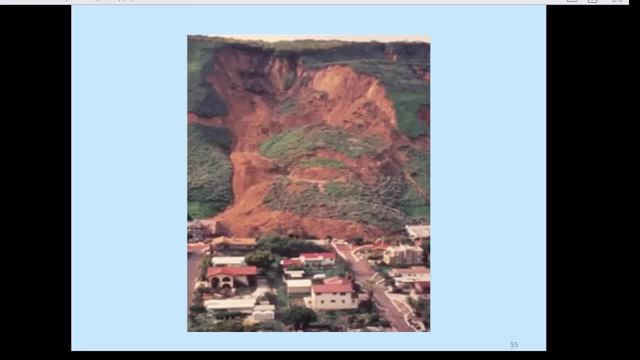 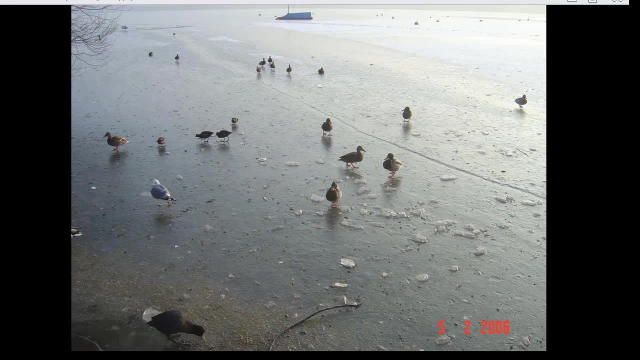 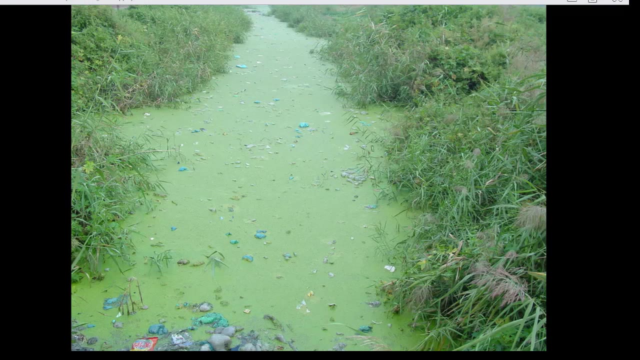 There's control everywhere, And then you may have extreme erosions. You may have extreme conditions where it blocks the flow of water into the river. You may have extreme pollution conditions, So a lot of things that happen in the watershed that you are not aware of. 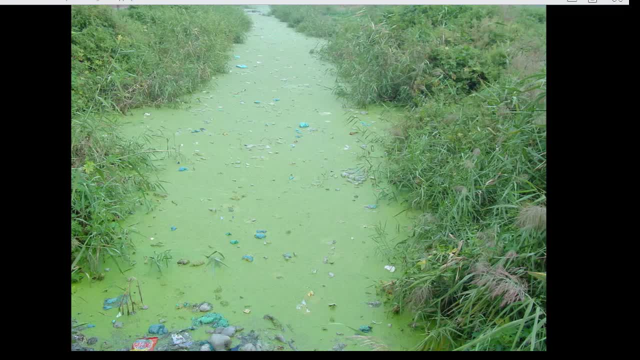 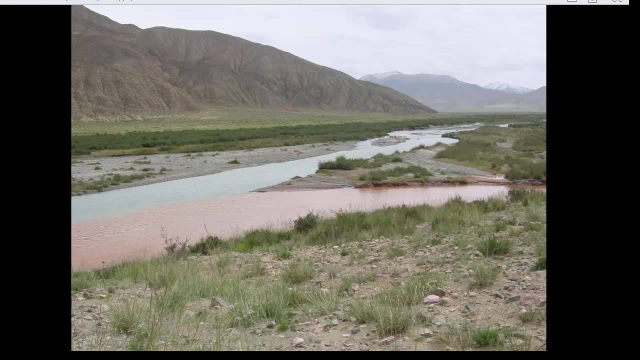 And then you try to model this watershed and expect a perfect result, So that doesn't happen. This is another interesting observation at the top of the origin of the Yellow River in China, where the rivers from two different sources join together to make the Yellow River. 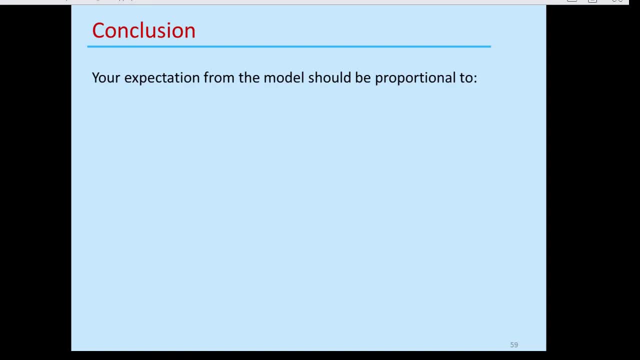 Now your expectation. in conclusion, Your expectation from the model should be proportional to your knowledge of the model and model parameters. Should be proportional to the quality of data and processes you put in the model. It should be proportional to the quality of the effort you put into model building. 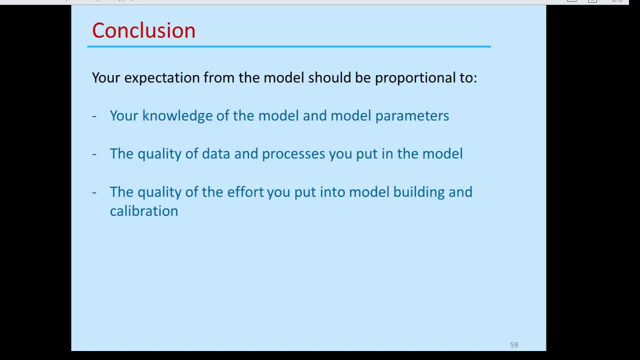 and calibration. So don't write me that I have two weeks to hand in my thesis and I need to calibrate my model in these two weeks. There is no way you can do that, So don't try to get also at the end. 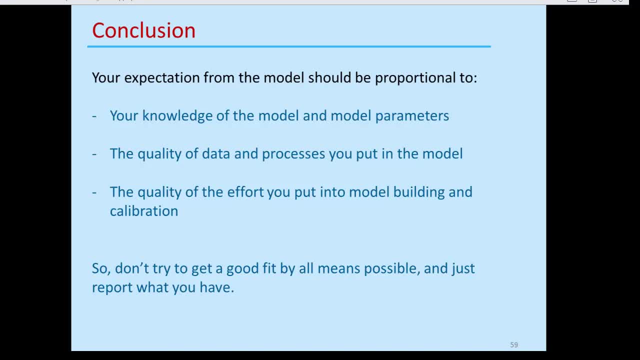 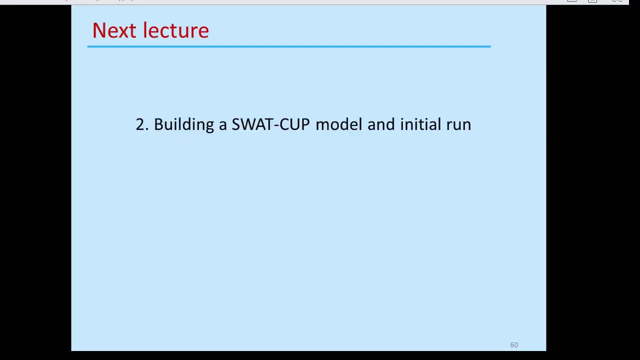 Don't try to get a good fit. by all means possible. Just report at the end what you have and that reflects your knowledge and that reflects the goodness of your data that you have put in the model. In the next lecture I will build a SWOTCOP model. 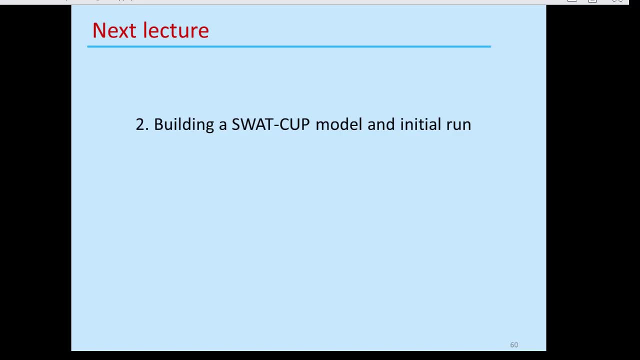 from the beginning using Texin-Out data and then we make an initial run and we'll see what we can do with that model after we see the initial run. Thank you.